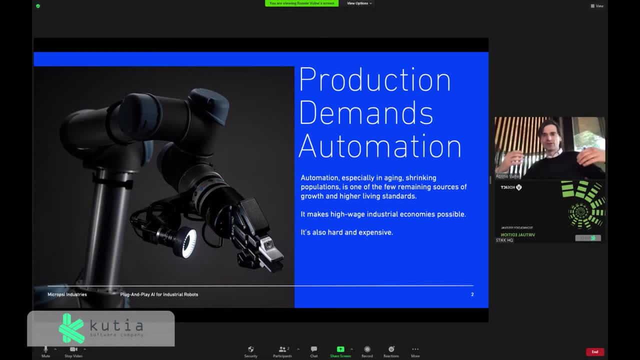 So, if you look at it from a macro perspective, doing automation- essentially using machines to do more with less effort- is one of the few remaining sources of actual economic growth, and that's where we're coming from. It also means if we automate- if we continue to automate, we can continue to pay high wages in manufacturing. 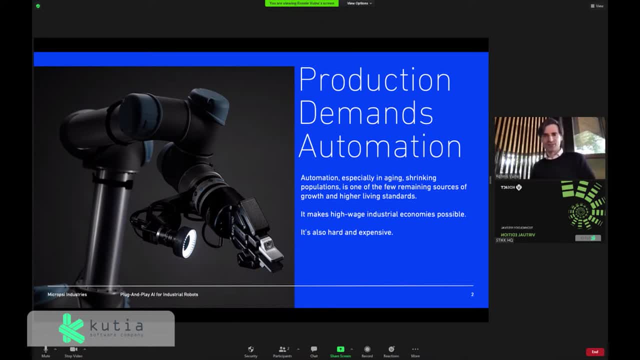 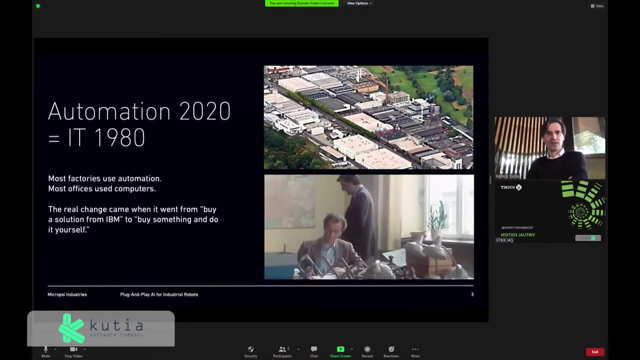 And it doesn't all go. So automation is super important. Production needs it, especially in the West, especially in Europe, and unfortunately it's also super hard and it's super expensive and it's super inflexible. And the way we look at it, automation- and that includes pretty much all of robotics- today is roughly in the same spot that IT itself was in the early 1980s. 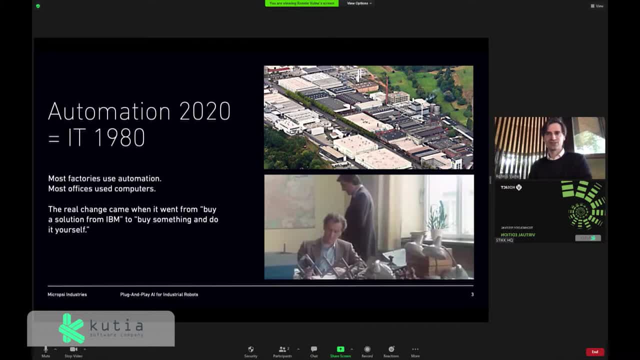 So you know people are doing it. It's not sci-fi future technology, it's there. but if you install robots, if you automate production lines to a degree where you know can't take away the humans from them, you're almost always looking at, you know, multi-year projects that are super expensive and need to be done by professionals and that's sort of in the way of adoption, right. 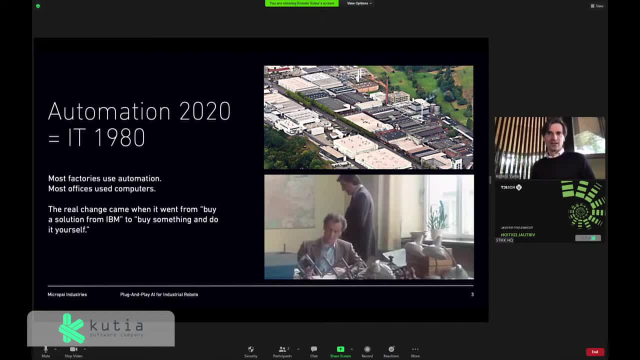 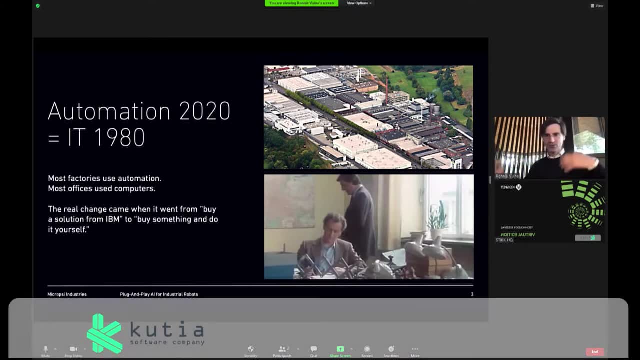 Because that makes you too inflexible, it's too expensive for most people, And IT was exactly like that in the early 80s. You needed to buy it from IT. People in white coats came and they were experts and then something happened, and what happened was the market moved from big expert projects to small units that essentially anybody could buy and it wasn't as good enough as what you would have bought from IBM or the other big suppliers. 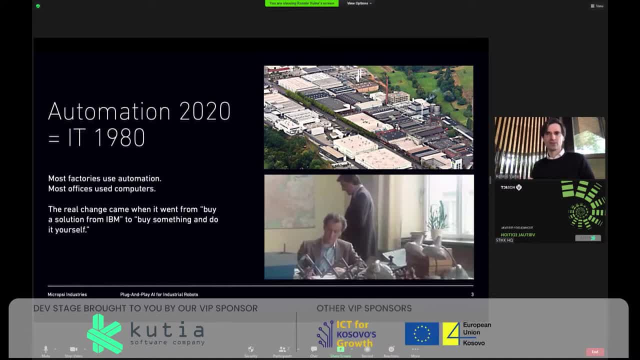 It was good enough So everybody could do it. And we believe that automation is pretty much in the same place. So you know, as IT had its PC moment, when it became available to everybody and got democratized because it was available in small units that everybody could use, the same thing is happening in robotics right now. 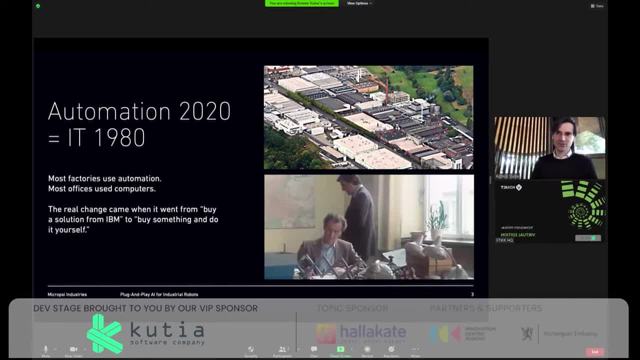 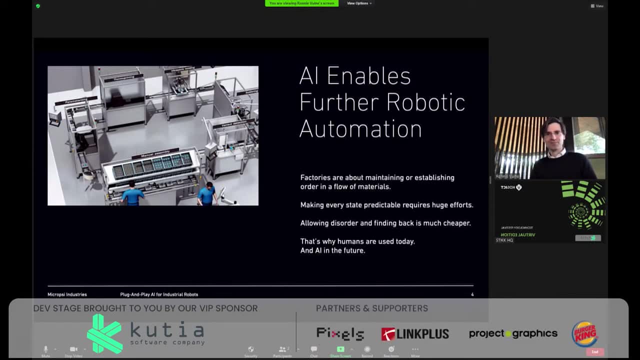 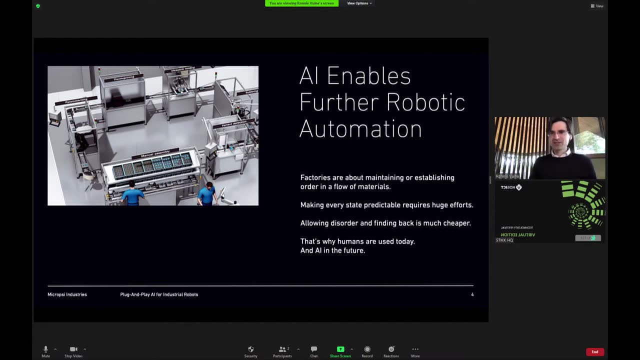 And we at Microsoft Industries believe we can contribute something to that change that is happening at the moment. So what's the specific role of AI when combined with robotics? So the way we look at it is, if you think about what a factory actually is, it's essentially a humongous machine for rearranging atoms, right? 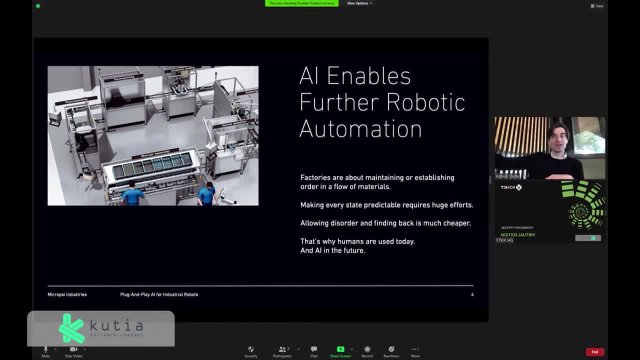 You put material in on one side and something that's more valuable than the raw materials comes out on the other side. That's what the factory does. It adds value by rearranging atoms on the flow, on the way of the flow of the robot. 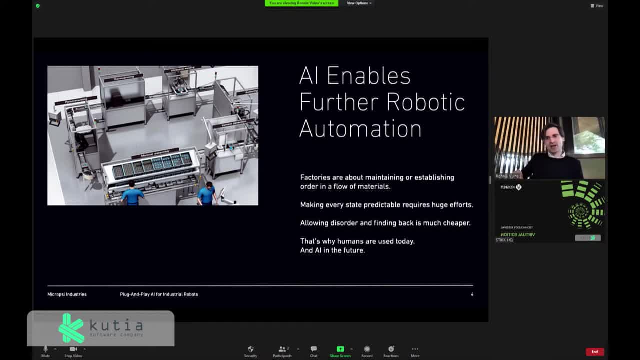 And that's what the factory does. It adds value by rearranging atoms on the way of the flow of the robot, And that's what the factory does. And that's what the factory does. You put the material through the factory And if you want to do that, and if you want to rearrange atoms, you sort of need to know where they are before you start rearranging them. 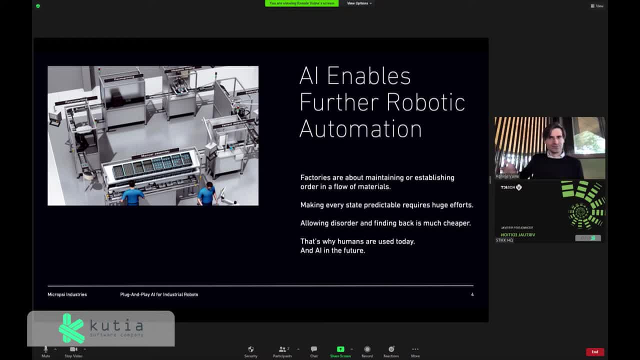 So everything needs to be properly and neatly ordered, And that, of course, is extremely expensive. It's less expensive if you're doing cars, because they're made out of metal and this behaves mostly predictably, so you know where your car is at any point in the factory. 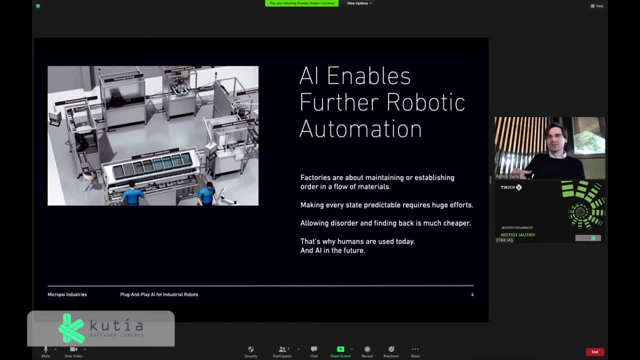 But for many other things it's a lot cheaper. many other things, especially if you involve cables or rubber or any anything that moves or is slightly differently shaped. knowing where all the stuff is in the factory is super expensive and usually can't be done today, and that's why you use humans. so because they're super flexible, they just you. 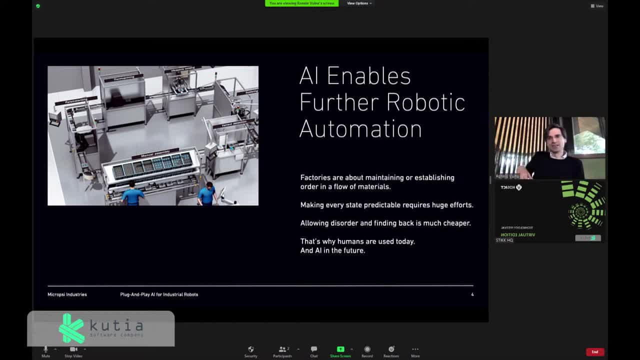 know, look at something and will know where to pick it up and how to handle it. so robots couldn't do it, because robots, or as any other machine, they're just a bunch of electrical motors and software and they need to know exactly where something is that they're supposed to handle or manipulate. 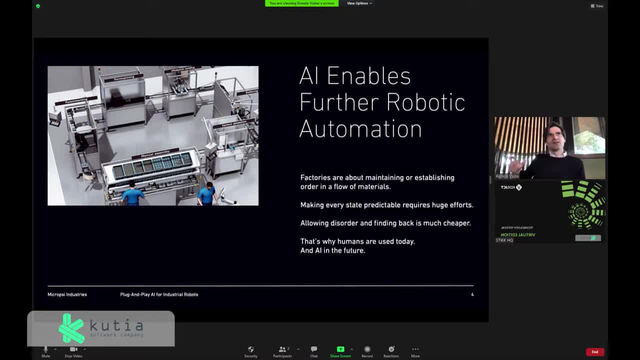 so today manufacturers, even in high-wage countries, still use humans to sort of allow a bit of disorder to happen because that's cheaper, and then use humans to find back and have them sort something from just a heap of stuff into a machine where it's neatly ordered and can be. 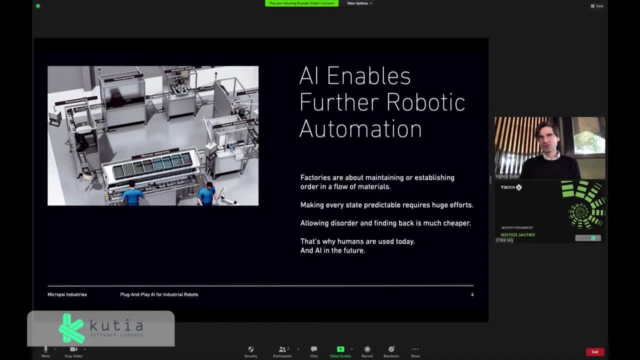 and can be processed. so today you use humans and if you want to move away and automate further, you need to use more flexible, flexible machines than specialized machines that can just do one things- that's robots- and you need to use a technology that's as flexible as humans to you. 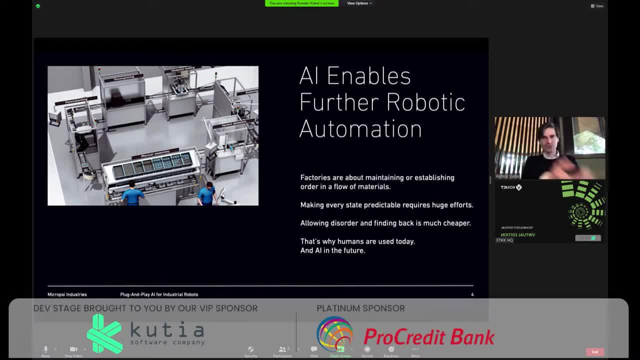 know, understand the state of the material that's coming towards the processing station and deal with it, and that would be ai. so this is why this combination of ai and robotics is so exciting, because it allows you to essentially automate further beyond what you could do before with the. 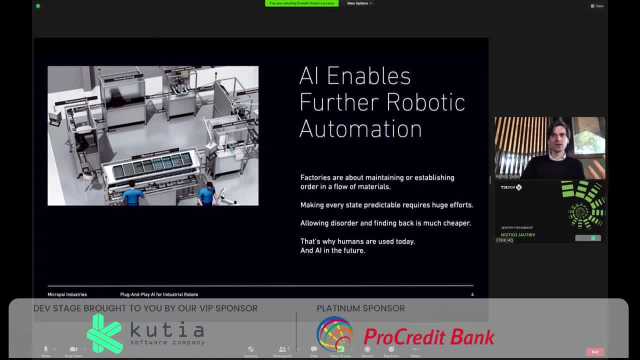 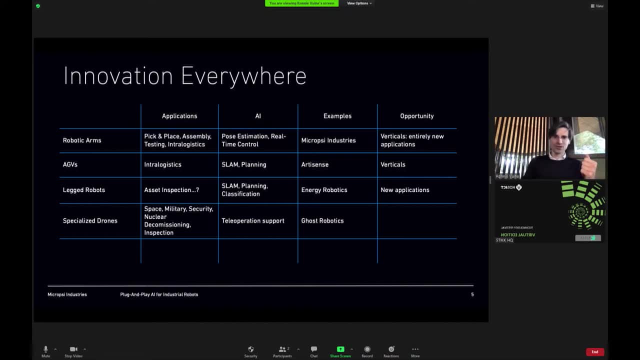 new technologies that, um you know, came into being in ai over the last 10 years. so i apologize for this slightly boring slide. um, it's- at least it's- boring looking, boring looking, but it's really packed with, um you know, a way of systematizing what's. what's, what's happening, uh, in the field. 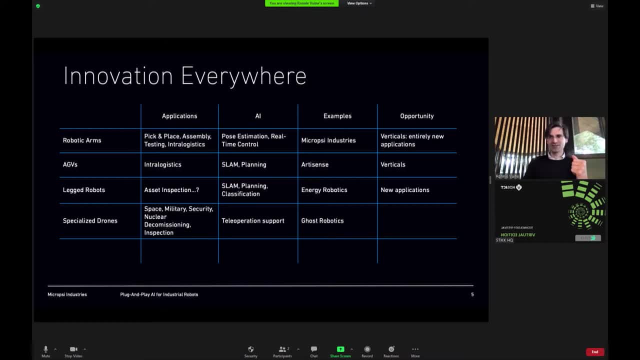 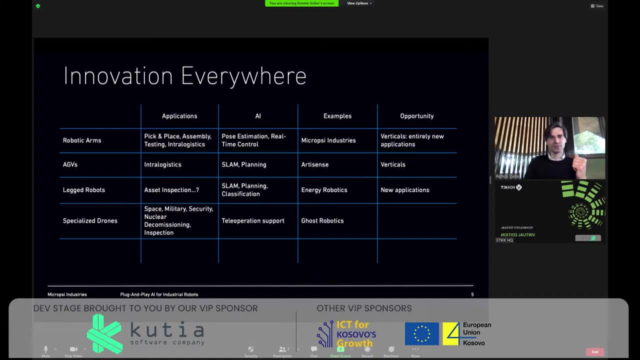 and we'll just go through it. um, and as this is online, you can maybe, in parallel, google the companies that i have, um, put in examples and look at what they're doing. so, um, on the on the left here i have um the types of uh robots where we see major innovation, uh currently and um, i mean. 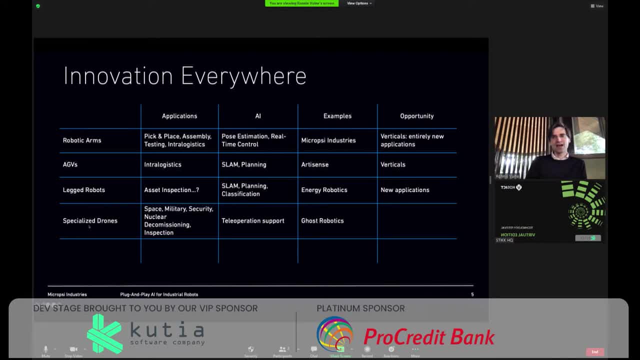 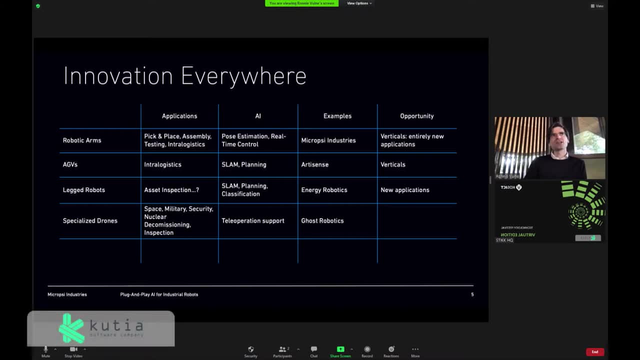 let's start. let's start from the bottom. um with you know highly specialized machines. this is mostly, mostly drones. so these are machines that are essentially custom built by robotics companies or produced at you know small scale for highly specialized applications like nuclear stationing, um space applications. or you have things that you can put in the iss and would. 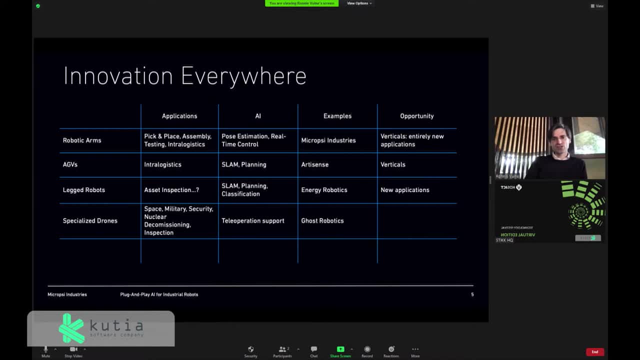 manipulate something there, um, some of the inspection cases, um, and there is virtually no ai in these, uh, in these, in these robots, uh, usually because, um, everything's so expensive and so high stakes, uh, all the time that you essentially want to teleoperate them. so if you, 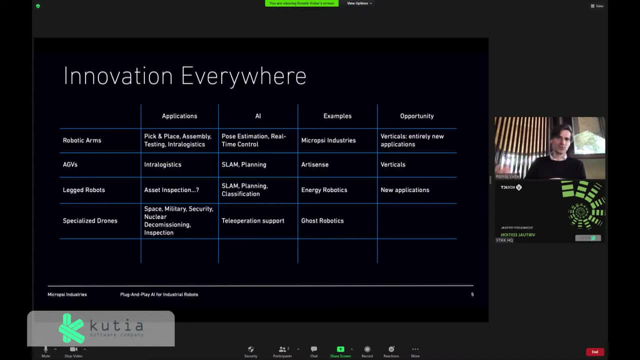 do any ai? um, it's usually supporting teleoperations. um, the one of the companies that is active in the field that is quite similar to one that you have probably heard of- the one you have probably heard of is boston dynamics. um, just got sold yesterday. i think again um one of. 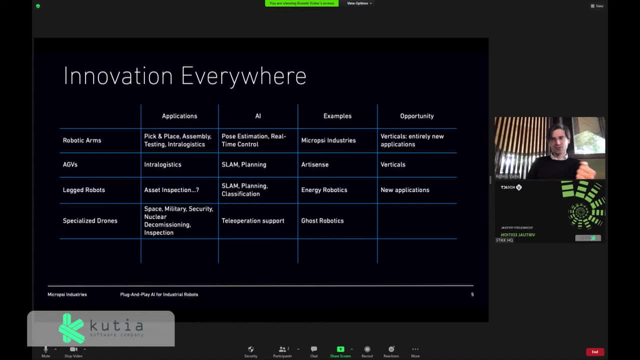 the one of the companies that's um, that's, you know, similar um in scope, but with a more clear focus than boston dynamics has, is, for instance, ghost robotics, and they're completely military. i visited them two years ago and if you, if you go there, uh, what you see is, you know, oil paintings. 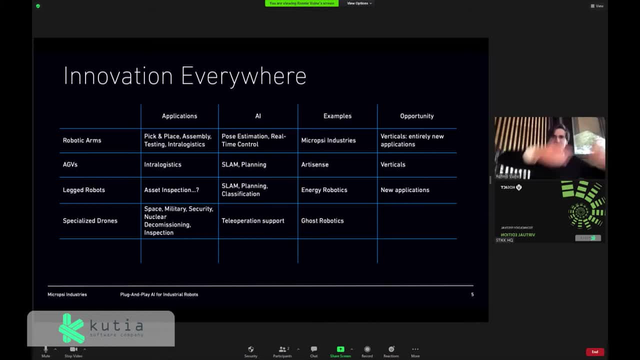 of people throwing four-legged dog-like robots and they're completely military, and they're, they're completely military, and they're completely military and they're completely into into houses so they can run around and scout if anybody's in there. so these are, these are, these are mostly teleoperated machines. um, because what you're doing is too high stakes. um, and too. 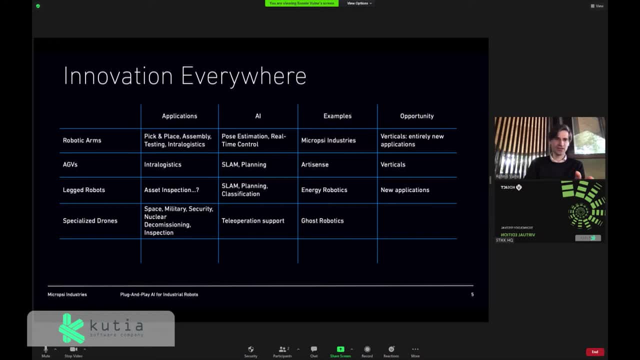 custom um to handle it with ai today, and then in the same field of legged robots um you, you get some semi-standardized applications um, mostly in asset inspection, and an example would be energy robotics, um startup, i believe, from munich here in germany. they essentially took a spot robot by boston dynamics. so again, something that 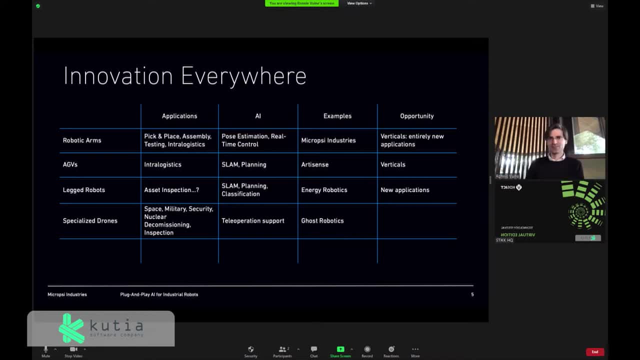 looks like a small dog, has four legs and is, you know, right in the center between being super cute and super scary. um, and they put cameras on top of that platform and they have it running around in a factory and just look at things. so this is mostly valuable in process industries. so where? 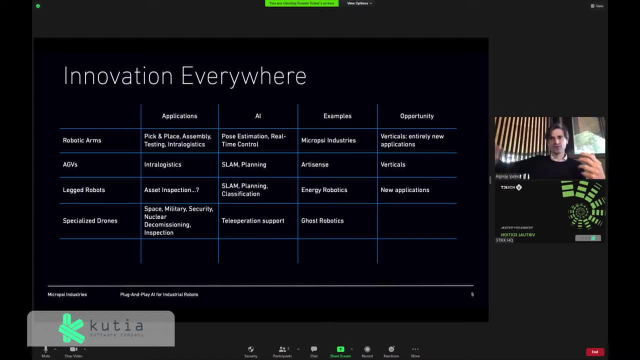 you make things with a continuous flow of materials, so you don't have discrete steps. so this means it's mostly pipes right, and you have lots of pipes to inspect, and today that's something humans do. they will just go along and see if they see any leaks or anything that looks worrying on those pipes, and the idea is to do this with robots. 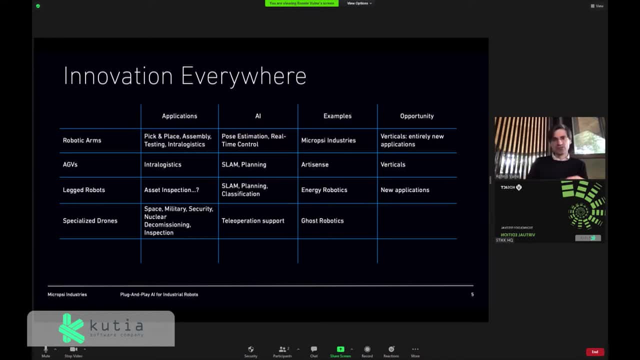 and to do it with legged robots. so, ai wise, what you need to do this is a bit of planning. so where do you go when? um, and you need a bit of simultaneous location and mapping slam, you need to be able to tell a good pipe from a bad pipe, so you have a classic. 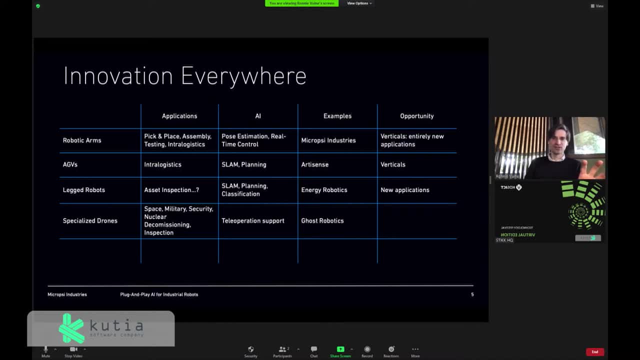 classification ai problem that you're, that you're also uh tackling um and uh, you know this is there must be more opportunities for doing things with those legged robots that are now available, um, beyond the acid inspection use case. i don't know um, but it's certainly worth looking into this. 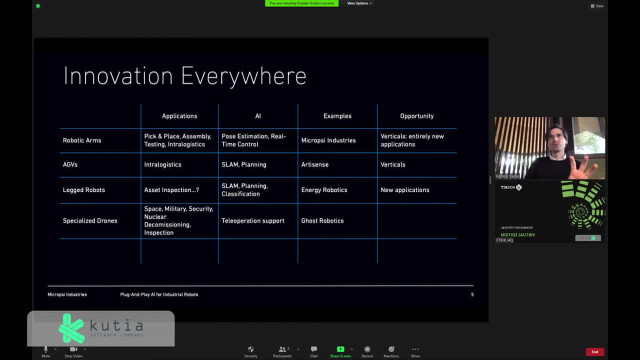 the platforms are now available. you can, you know, bring unmanned vehicles into rough terrain now, because we have four legged robots that can, you know, climb a steep hill or be out in the woods or be in any form of terrain that a wheeled robot couldn't go through, and we're not really seeing the applications there. so i think 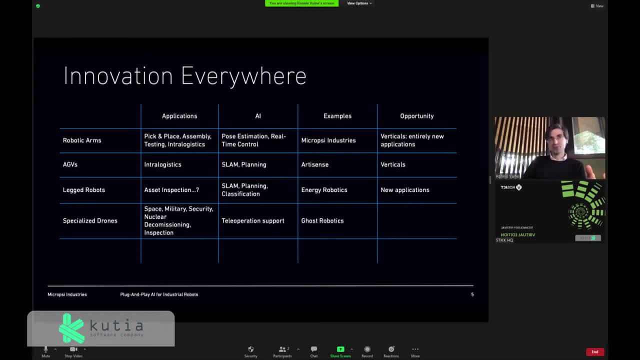 lots of people are looking for ideas of what to do with platforms such as ghost robotics or boston. dynamics and energy robotics are an example of adding software, adding ai, to do some thing useful with these platforms beyond the tele-operated use cases that you get from the you. 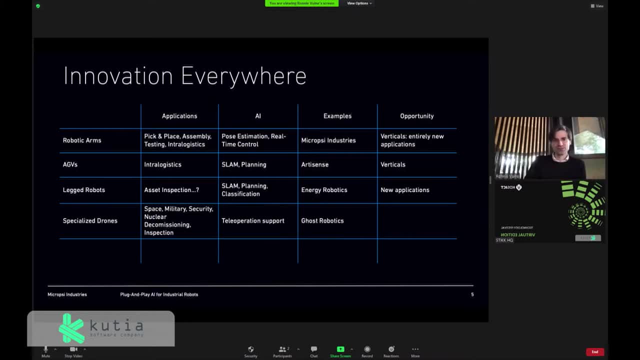 know super high stakes fields. and then, of course, the huge fields are autonomously guided vehicles, agvs. they're mostly used for intro logistics, moving stuff around in warehouses and factories without people needing to know where they go. this again, ai wise, is mostly a slam problem. so you want. 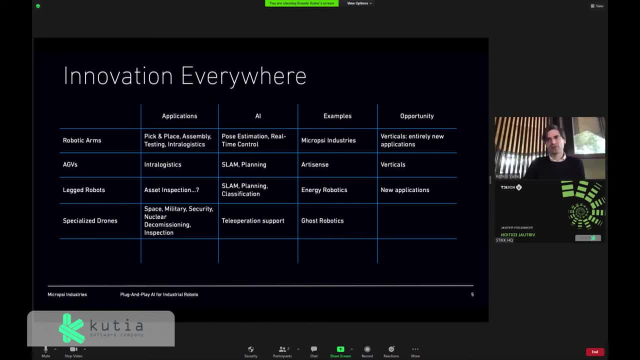 the robot to be able to create a map of where it operates. and you want the robot to know where it is on the map so it can sort of make a plan and, and you know, find a box of metal parts and take it to a machine where a robotic arm will handle it later on. um one of the more spectacular examples. 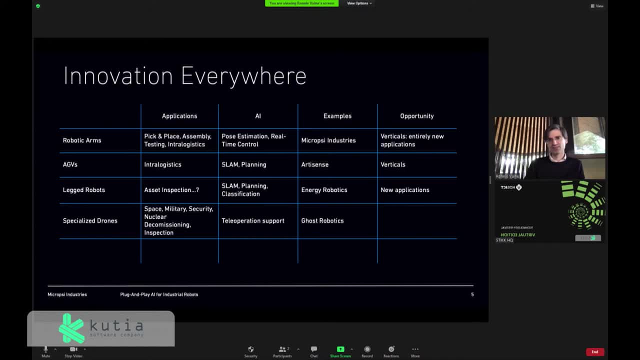 of really good um slam algorithms is done by artisans, again in munich. they're also a bit of a? um active in the automotive space, because of course you know if you can drive an autonomous forklift around the factory. this use case is very close to driving an. 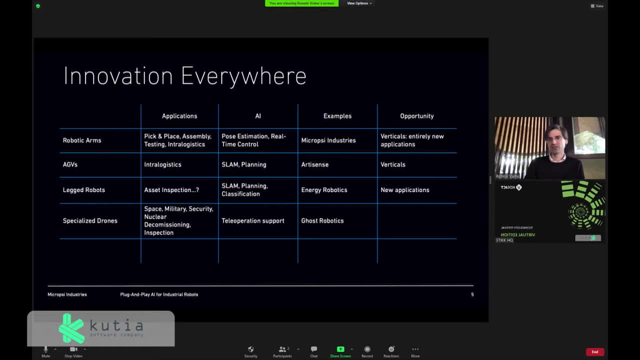 autonomous car around the city or at least a parking lot. so slam really matters, and artisans is a company that does this really well. they have really cool demos. the opportunities in the field are again in just vertical applications. agvs come in all forms and sizes from very small platforms that essentially carry a shelf around in a in an amazon. 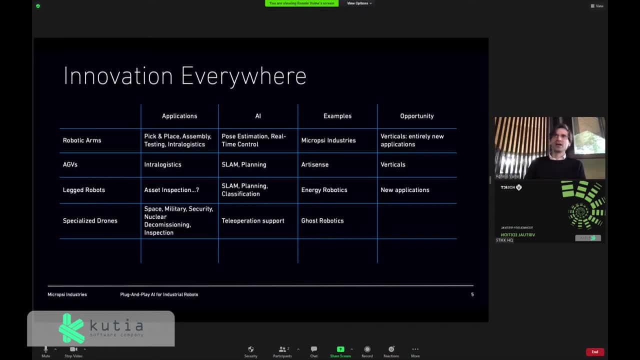 warehouse to forklifts, and one of the more interesting applications i have seen was a specialized agb that was able to pick cans from shelves for distributing drinks. and if you want to do data scale, it pays to have an agv, essentially an autonomous forklift that can drive up to a shelf. 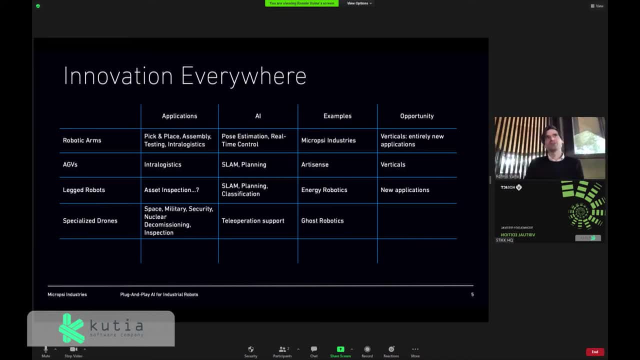 get individual cans or a pair of cans, and then you can actually carry a lot of the stuff in the factory pallet of drinks for delivery. And then, of course, finally, there's the space that we're active in and that we find most exciting, which is robotic arms. So six electric motors in metal. 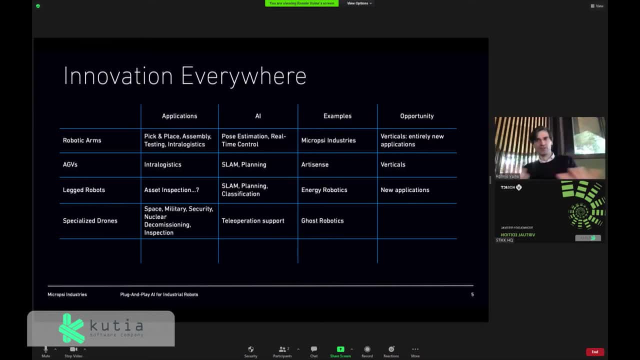 tubes bolted to a table that can manipulate and build things. The applications that we're seeing there are mostly pick and place, So you have a part and it's in a box and it needs to be put into a machine for some grinding or some further processing And then it needs to be taken out and 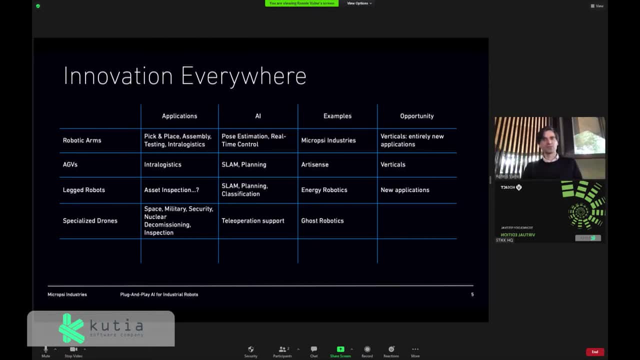 put in a conveyor belt and taken elsewhere, or on an AGV and taken elsewhere. So these are pick and place applications. You have assembly applications where you really clip things together or screw things together. We have testing applications where you've done the clicking or screwing things. 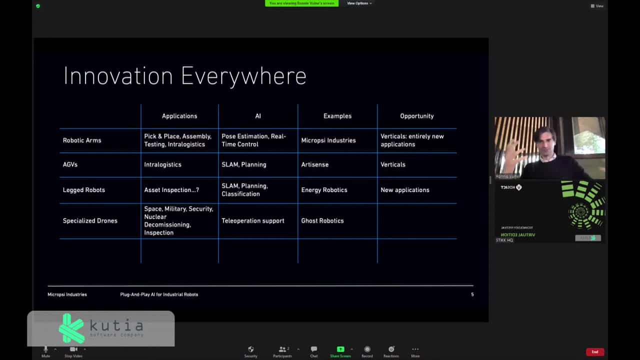 together and then you want to know: does it work, Is it in a proper state? And again you have applications where you just need to move stuff From one table to a second table or from a table to an AGV or vice versa, And the AI problems in. 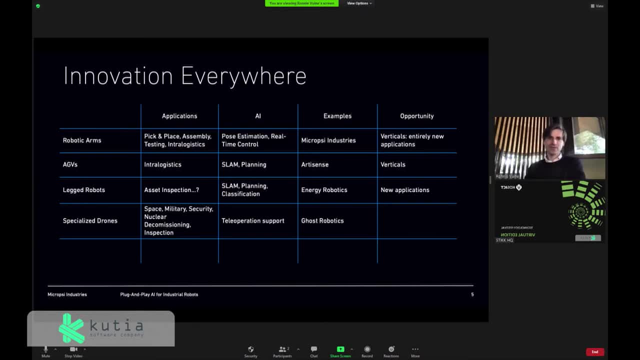 that space and that's certainly where I'm most familiar with are. so we sort of divide the market into two big types of AI approaches. The first one is you want to move a robot to a piece or to a machine and you have essentially a 3D model and a 3D camera and then you fit the model. 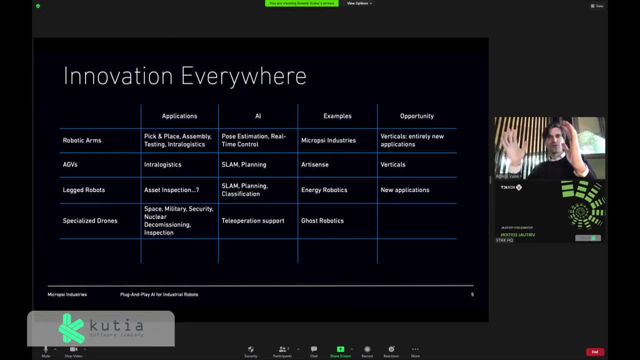 into a machine And then you have essentially a 3D model and a 3D camera and then you fit the model into the point cloud you get from the 3D camera And then you have a 6D pose right Three: 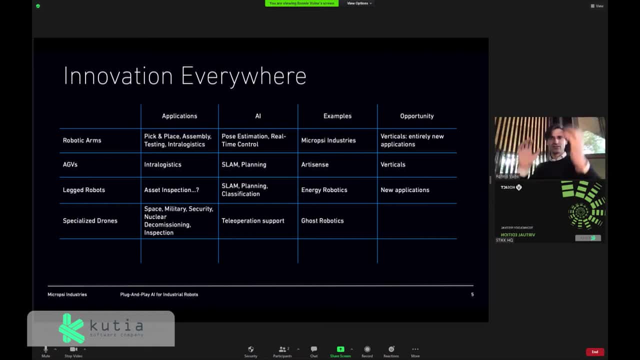 transitory dimensions and three rotatory dimensions. You have a 6D pose for where the object is and then you move the robot up to the object and you move it relative to what you've measured with your 3D camera and your 3D model of the object you're handling or dealing with. And that's pose estimation. 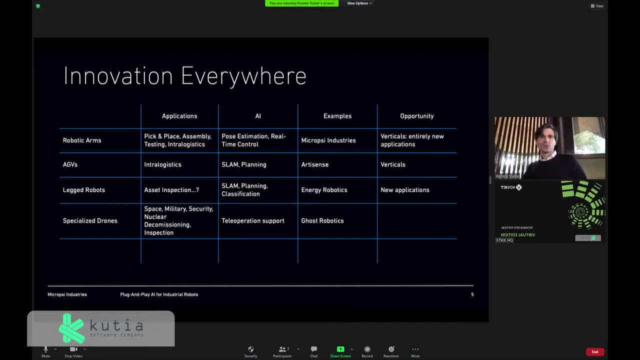 And then we take a slight different approach. We do real-time control. So just to illustrate this: if we, as humans, plug in a cable into a phone for charging the phone, we don't have a 3D model of the phone in our heads. 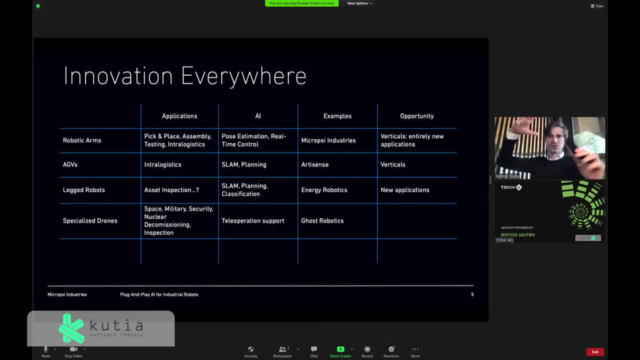 not even close And we don't have a full 3D picture and we don't sort of take a single measurement where we fit a 3D model into the point cloud that we get from our eyes. What we do is we just move. 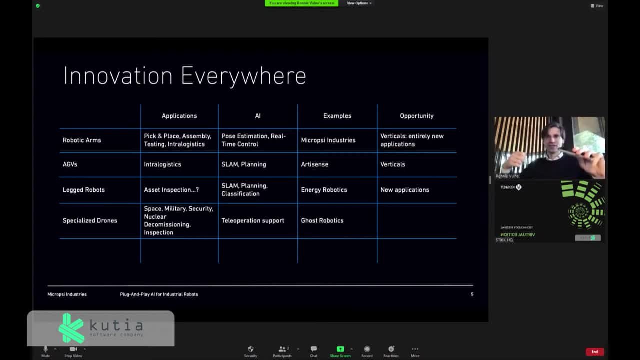 towards with the cable. we take a 3D model and we plug it into the point cloud And then we move towards with the cable in one hand and the phone in the other. we just move towards each other and wiggle a bit And as we get closer we see how we need to make small corrective movements. 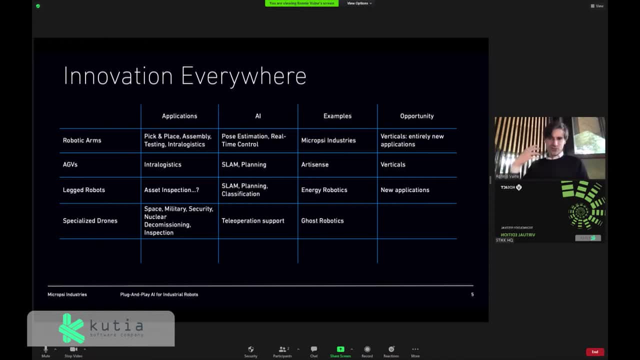 to get the cable in And this real-time control is fast making decisions from visual and haptic input, where you don't try to find an absolute pose of what you're handling, but just relative movements that you need to make to end up in the right position is what 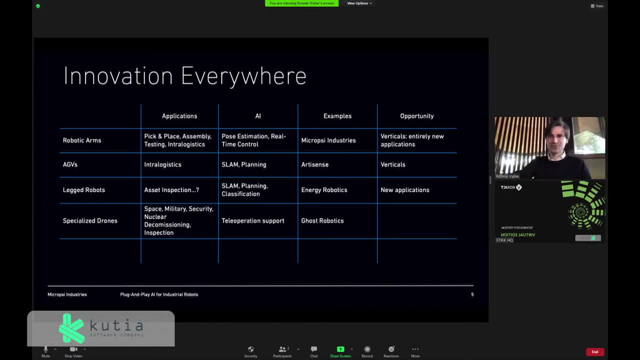 micropsy industry does, which I have, which is a convenient example for a cool AI and robotics company. The opportunities there are not in the AI itself. I would say, of course you can always beat us, but the opportunities are mostly in doing things with existing robotic arms and existing AI systems, That you can generate different types of interactions between robots. you just need something to add in. So these folks that I mentioned before has the right bouncing in the same direction, a better不同 from what they used to do, a same Independents. built which is being the same two which is being applied in security, but really slightly different. it can have a very complex interaction So you can not always be able to execute and adapt. You kad store things shown, multiple of them, in a row. you can use a different type of Gesetzent for stitched in the stage, for example. We 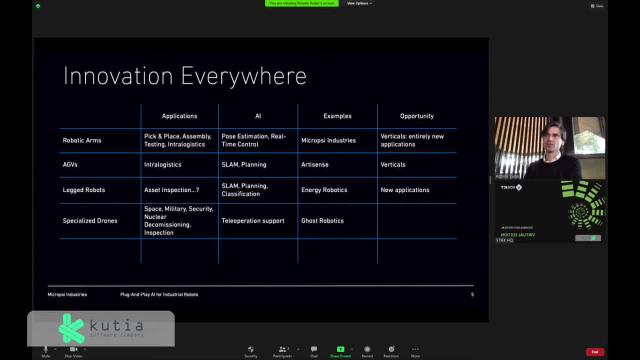 so far nobody has thought of, And some of the more interesting concepts I've seen are in construction or, you know, in picking things in hospitals or making pizza with robots and an AI system that can, you know, handle the variance that you naturally have when you're assembling. 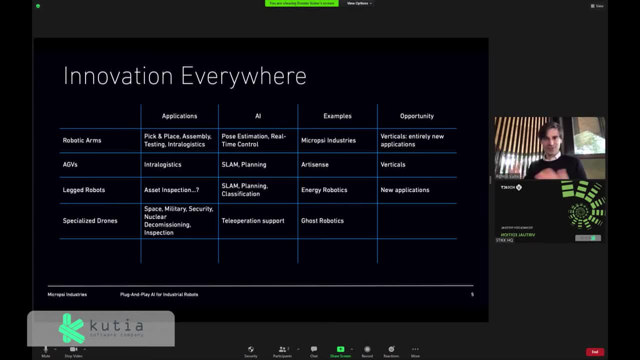 something that's made out of food never looks the same, So you never know where the atoms are, And I think there's going to be a whole wave of new companies, just like you have in the case of leg robots, where people take existing platforms, take existing AI systems, take existing robotic. 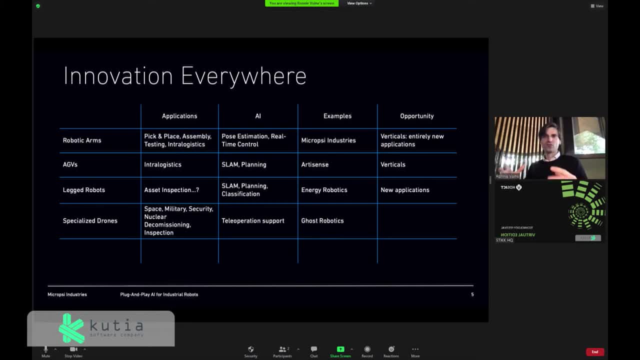 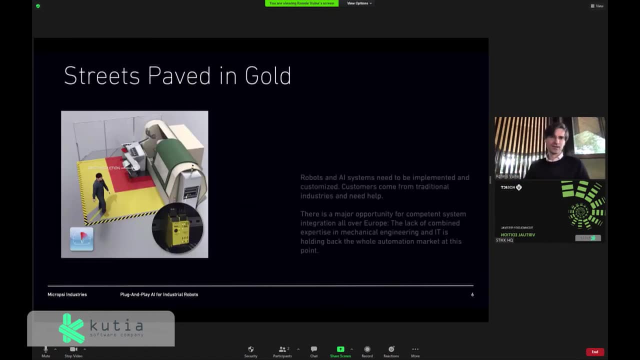 arms, put them together and do something that so far couldn't have been done with machines and would have had to be done with just human workers. And then there's one major opportunity- and I'm only half joking When I'm saying streets paved in gold on the, on the title of this slide. there's one major 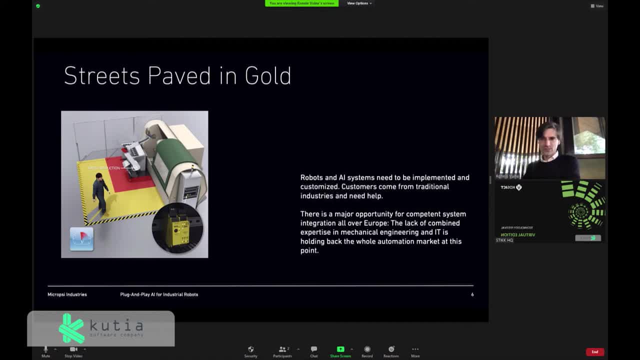 opportunity in system integration, especially in production and logistics, because all of this is mostly new to people who run factories. right, They're not AI people. they don't know what they're buying in many cases, or they will have one person who sort of knows what they're doing. 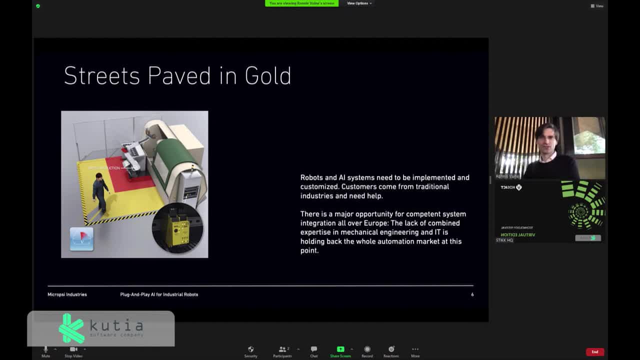 But it's really not common knowledge in the organizations of people who want to automate. So all these new technologies are now available and you could build machines and factories from them, but people really don't know how to do it And I don't want to learn it because they're running. 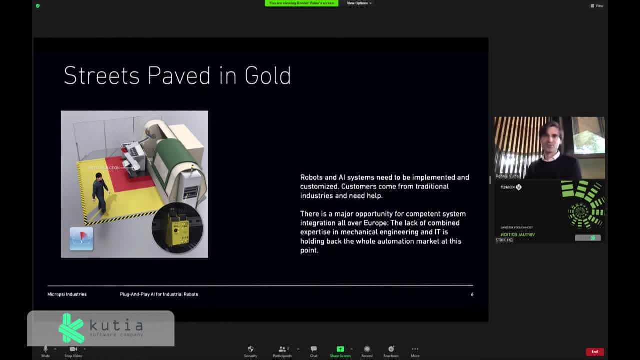 factories that make- I don't know- coffee machines, and they really don't want to be experts in applying AI to their systems. So the whole market- and it's certainly true for us and for the robotics guys who make the hardware and for many of the component makers who make- 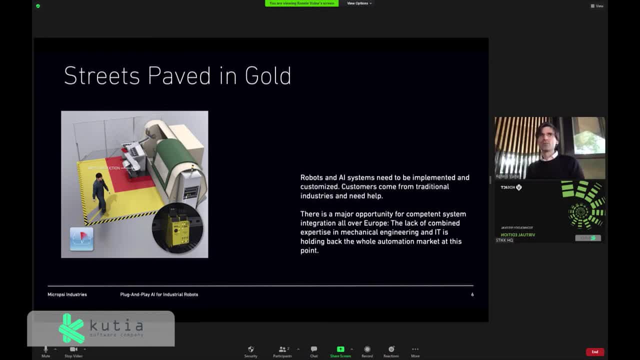 you know the grippers and all those things everybody pretty much feels held back right now And that means there would be money to be made if somebody could do it by the lack of competent system integrators, people who know enough mechanical engineering and enough IT to be. 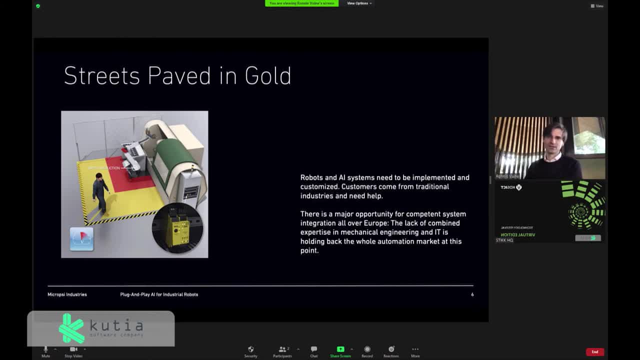 able to go into a factory, deploy these systems, get some money for it and then do it again for somebody else. Pretty much the whole market is frustrated because two few people know how to do it and can actually pull it off and do it reliably. 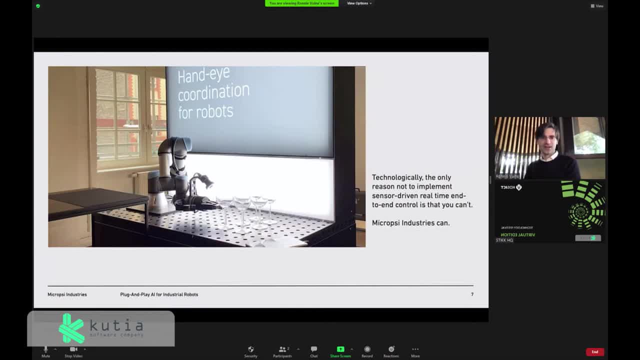 Okay, And then let me just show you some of the things that are possible now, At least one demo I have brought here. It's a Microbes Industries demo And it sort of highlights the specifics of what we're doing. The only reason to not 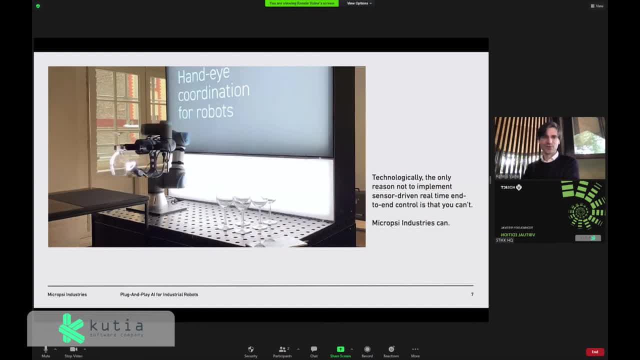 to not do what we're doing, which is real-time control over the pose. estimation is that you can't, and it's sort of easier to do that. So here in this demo we have like six wine glasses just on a table. They're in a rough order, but really nobody has ever measured where they are precisely. 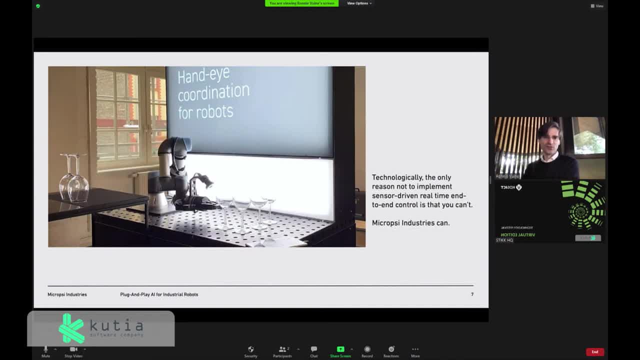 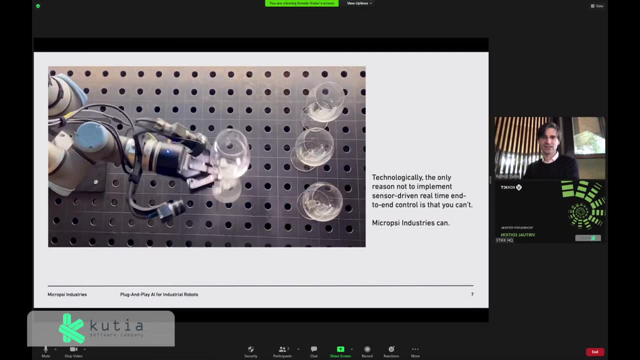 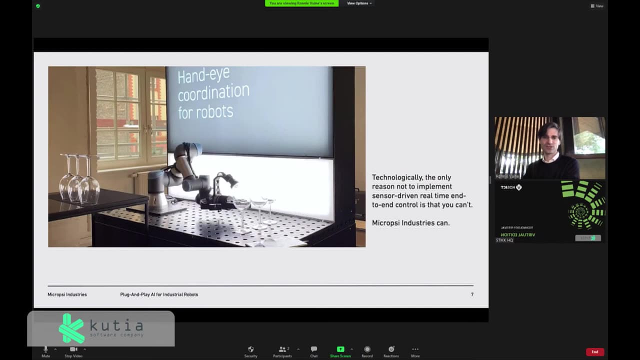 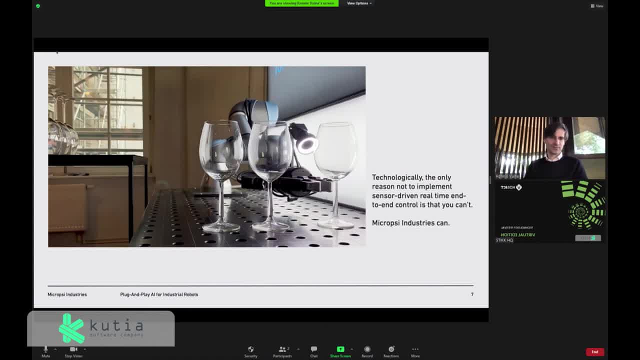 This is driven by our system. If I can, I pause this. Yeah, I can pause this. So if you, if you, if you look at this at the assembly, here you have a small robot by Universal Robots, Then you have a gripper by Robotique And then this contraption here, this is a camera. 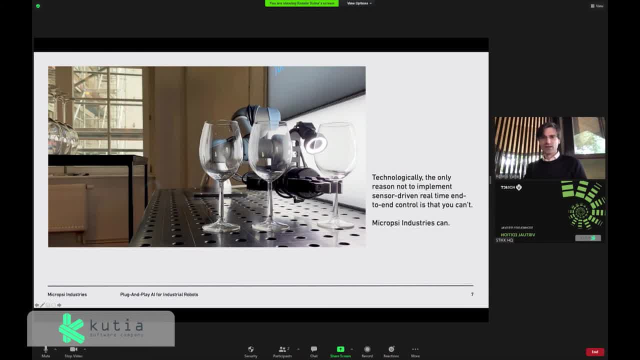 and a 3D printed camera fixture, And this camera is essentially driving the real time movement that we're making here. So, at 20 Hertz, this camera will shoot images, deliver the pixels to our AI system that has been trained by a human to to know how to move. 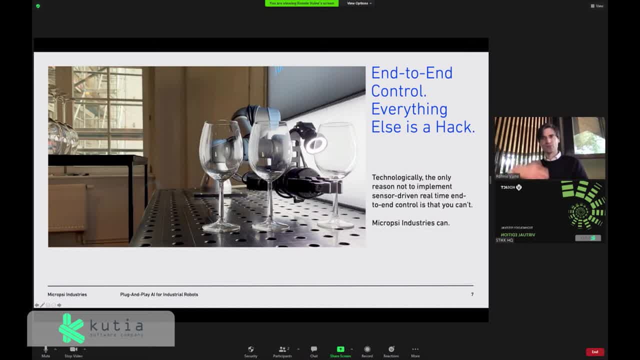 and then guide the robot 20 times a second with new instructions for the robot joints, how to, how to move, And that allows you to be super flexible. So you don't, you know, if you, If you, this is a real application somewhere in Nordrhein-Westfalen. 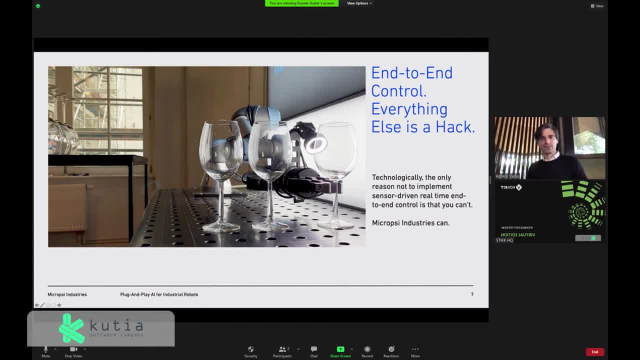 If you have a company that makes those glasses and they are just on a conveyor belt but they're sort of semi-ordered, they're never in the same place, Even if you have a hard computer vision problem like this, where you have reflective and translucent. 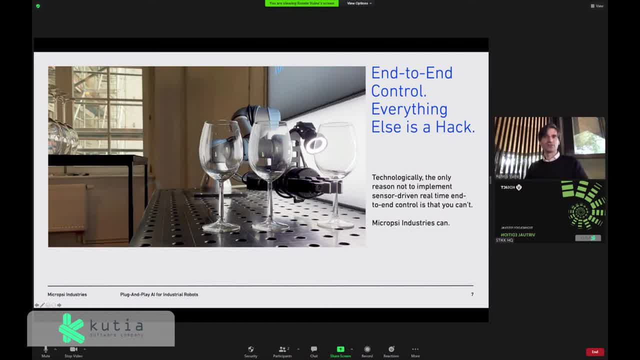 surfaces. you can pull this off and pick these glasses up and put them in order on the other side. The application, by the way, has been trained by salespeople, So this is not something that we custom built for this client. It is really just a product of our system that somebody trained to perform this. 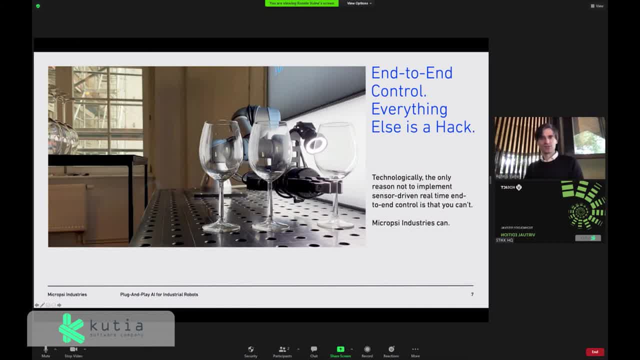 And training in this case means generating the data, which means guiding the robot by the wrist as you would guide a human. This is how you pick up the glass while the camera is watching, And you do this for two afternoons, and then it'll be able to do what you're seeing here. 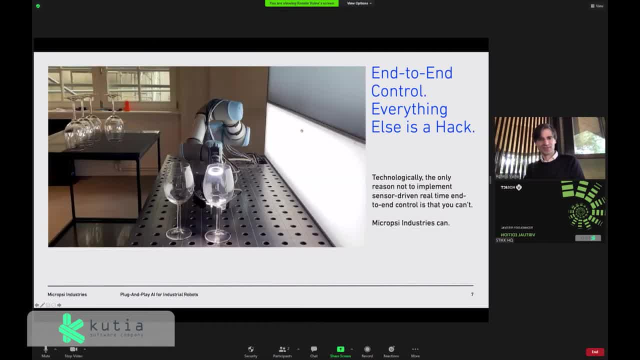 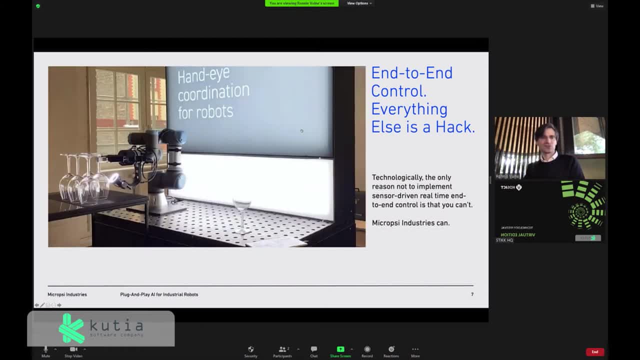 I'll just let that play out. Yeah, the range of applications is really, you know, from picking glasses to testing refrigerators, to putting metal rings into machines. We're really you know what a robot can do and where you have a bit of variance. that. 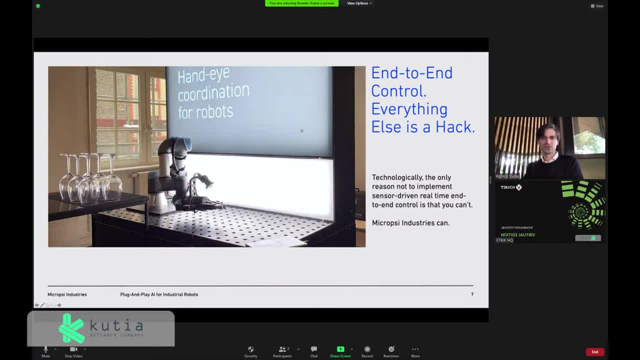 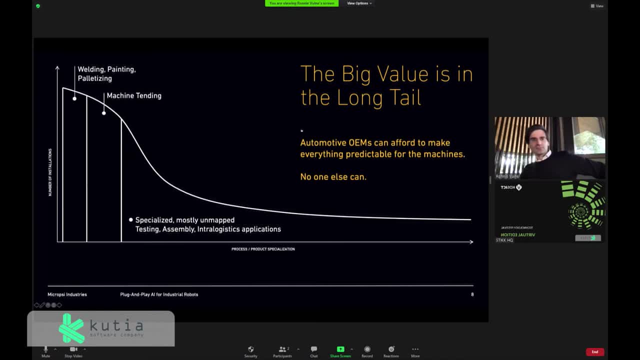 you need to deal with. you can train our system to handle it. Okay, and then a last word on the economics, The economics of it all. if you do anything like this and if you're active in the field of AI-driven automation, it's very easy to get carried away by. you know what the industry 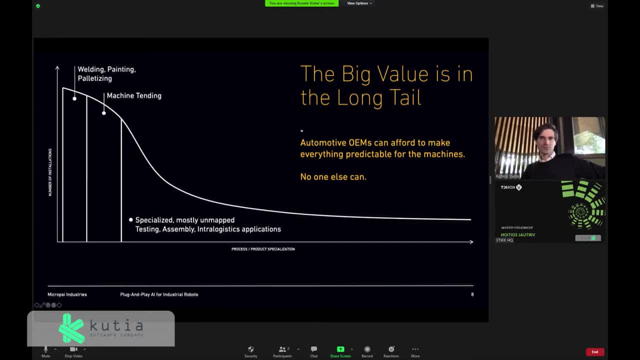 has been doing for the past 40 years. Robots have mostly been bought by automotive and, to a slightly smaller degree, by suppliers of automotive Metal companies. And then a bit of logistics. And they do these high value, high number of standardized deployment applications like 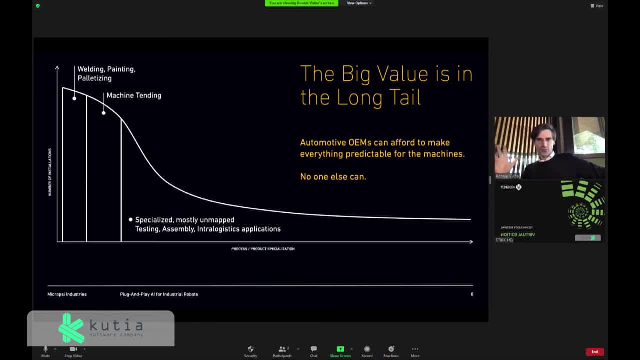 welding, painting, palletizing. That's where you would see robots when you just go to a factory today. So this is the classical market and has been served by the likes of KUKA and ABB and FANUC and some of the Japanese player, Kawasaki, for many years. 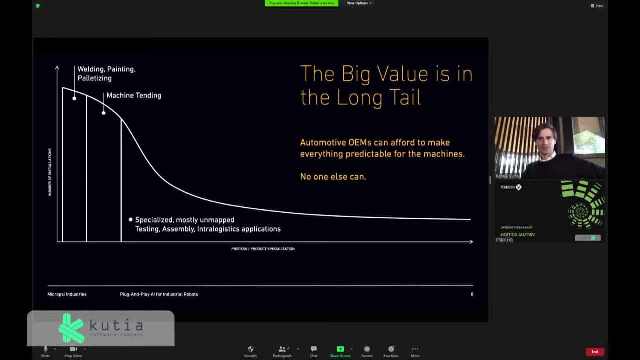 And there's Virtually nothing to be done there. right, This has been optimized for a very long time. It's pretty much perfect And there isn't much opportunity in that space. But what has happened over the last couple of years is that smaller, easier to handle. 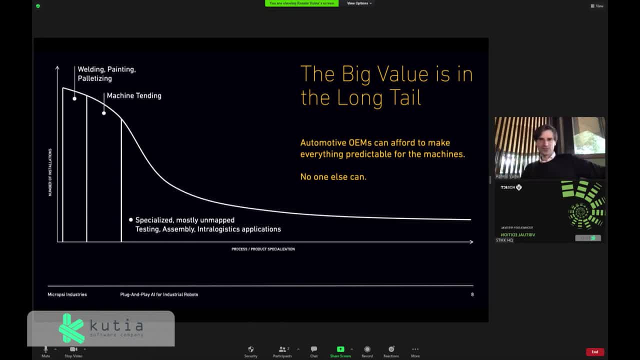 safer and cheaper robots have become available, For instance from Universal Robots, who we like to work with, And they have been deployed by people who couldn't afford These applications before. So new players, smaller factories or factories that didn't have any welding, painting or 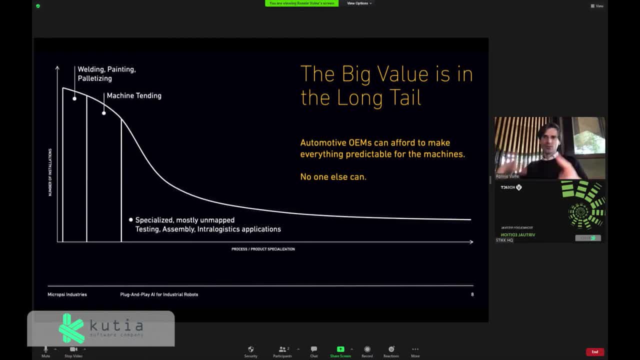 palletizing applications sort of started to put robots next to their existing specialized machines to just tend to the machines, just put parts in it, pick them, put parts in it. And that already is a large market And Universal Robots catering to that market has been growing with crazy numbers for a 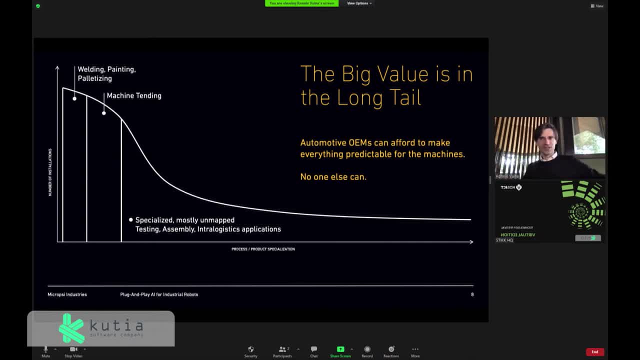 couple of years. And this is This is still you know, without any AI in it. This is just. you know where the part is, you know where the machine is. you take the part from A to B. A and B are well known. 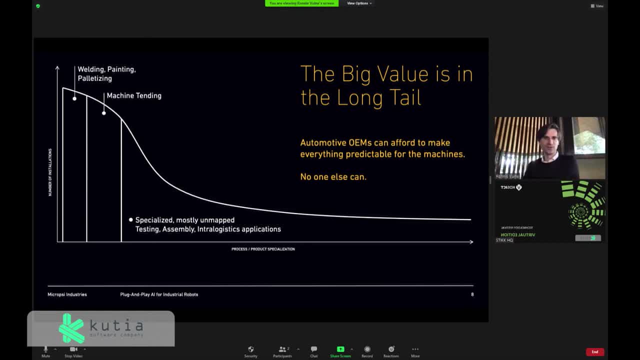 And you just program the robot to deterministically make that movement. And now what we're now seeing- and that's really what's enabled by the availability of AI in the space- is that you can go into the real long tail where you have applications. 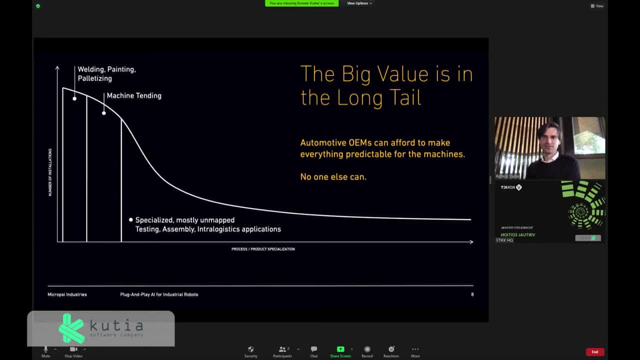 that really nobody knows about, right, Nobody in any research lab or, you know, on a whiteboard in Berlin we don't have it- has a list of applications that are super specialized, that are somewhere out there And they're essentially just in one or two or three or five factories, but they're not big. 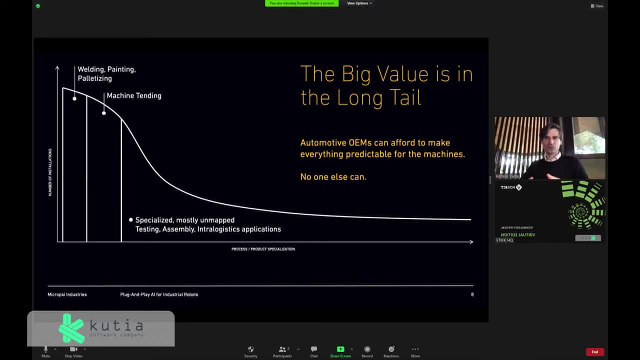 enough to go after for the traditional players who try to solve, you know, vertical applications that they know about. So these are these specialized, mostly unmapped applications and testing assembly and inter-logistics, And just to name an example that I always use, that you know I've been. 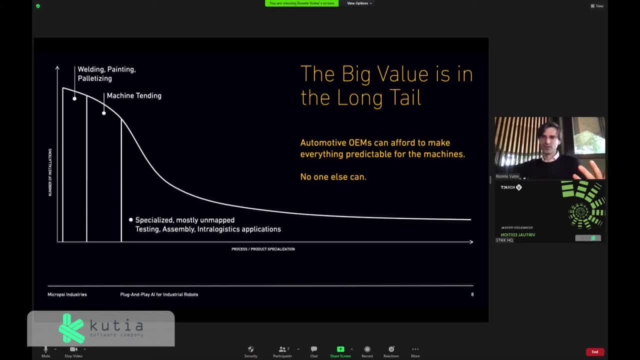 talking about. you know, I didn't know existed until I walked into that factory and people showed me There's a company in southern Germany and they make magnets for closing rubber tubes that go into coffee machines. So four people in the south of Germany make these for essentially any coffee machine. you 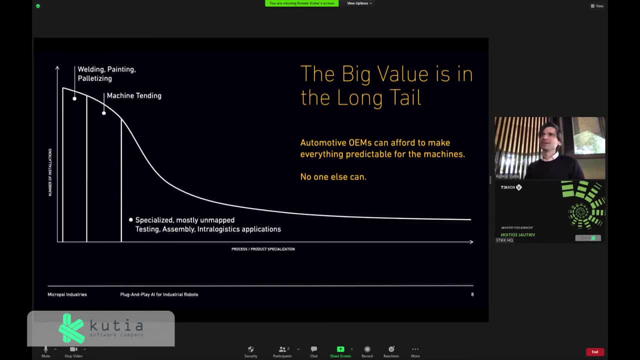 can buy from a German company And the applications there are about inserting some fiddly cable into a round part And it's just too special And you have the big guys to care about. So there's no standardized machine that can do that. 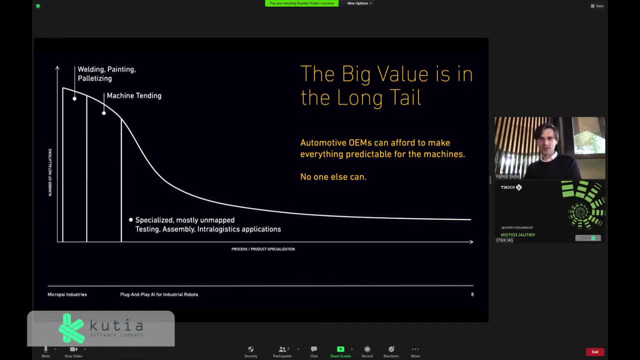 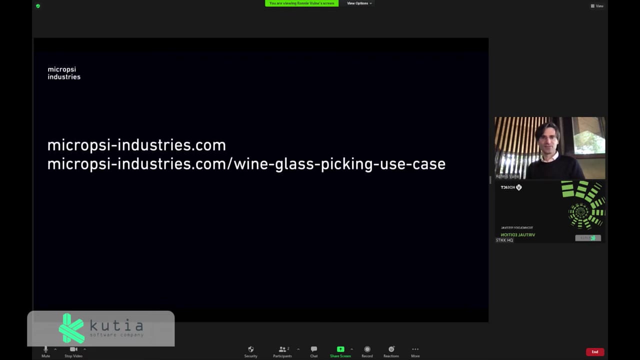 So your options are: either you still use people or you use customizable, customizable AI and train a robot to do it with a product such as ours. OK, so this is all I. this is all I had. This is the URL where you can find out some more about us, or the wine glass picking use. 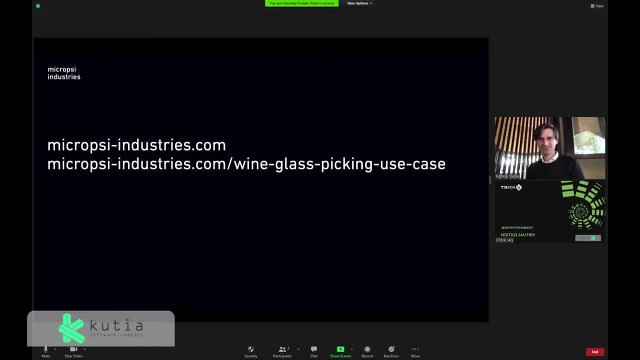 case, And I introduce thanks for your attention. I think we have 10 minutes for Q&A. So, yeah, ready, ready to answer your questions about us or anything that I mentioned during the presentation, And then let's see if I know enough about to give answers. 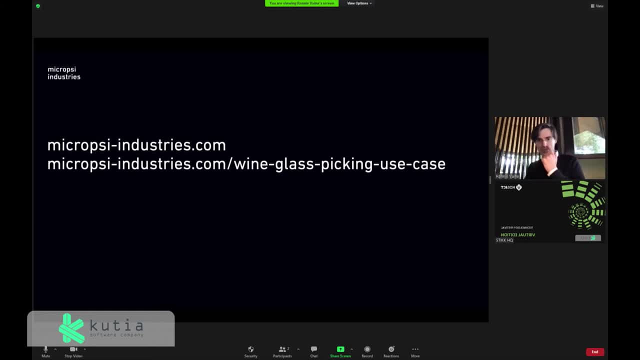 OK, While we're waiting for questions, I can also just maybe bring up a couple of videos So we're not bored while we're waiting, I think I need to go ahead and show you something. OK, OK, All right, So we're going to go ahead and show you some questions. 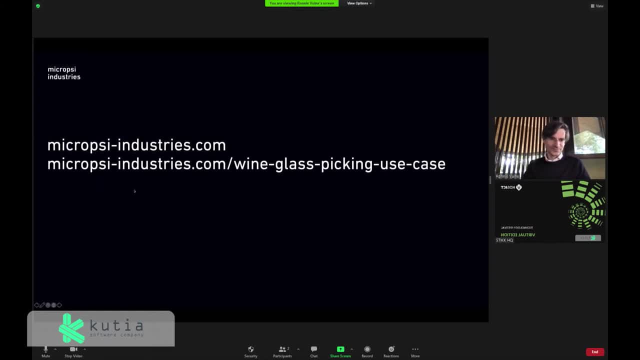 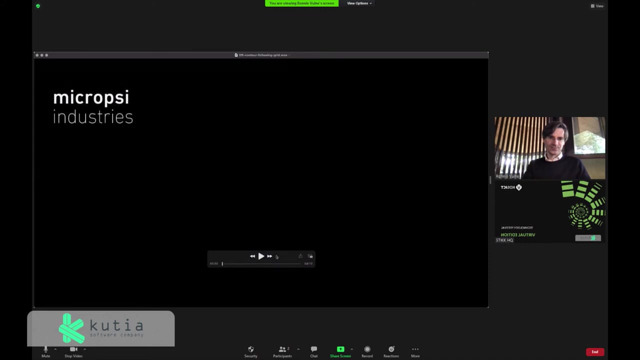 So I'm going to switch from my presentation to a video again, essentially just showing off with something you can do now with AI and robotics. This is an application where we needed to follow a very delicate grid structure on a structure that's made out of carbon. 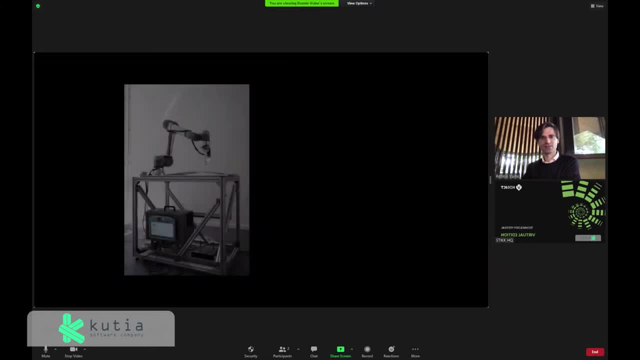 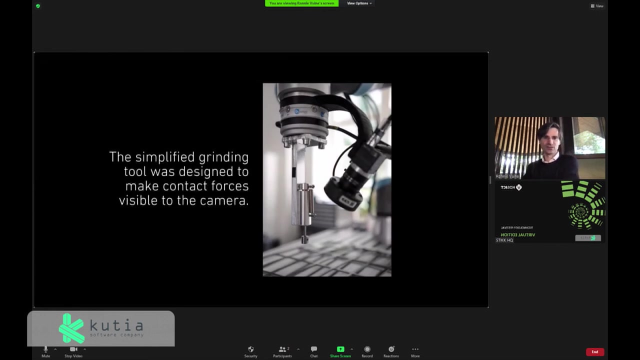 This isn't the full application. The full application is us guiding the robot to a point where it would first do very tender abrasive grinding And then there would be We put some glue on the structure that you now see in the background of that video. 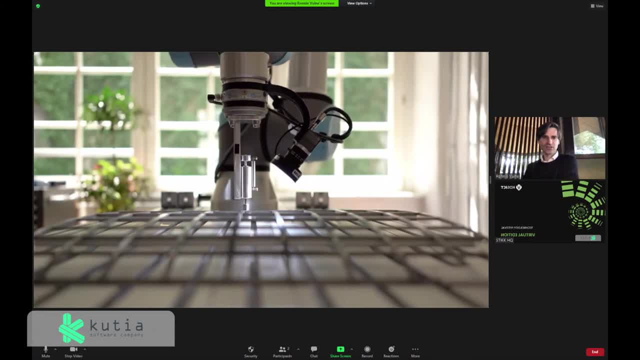 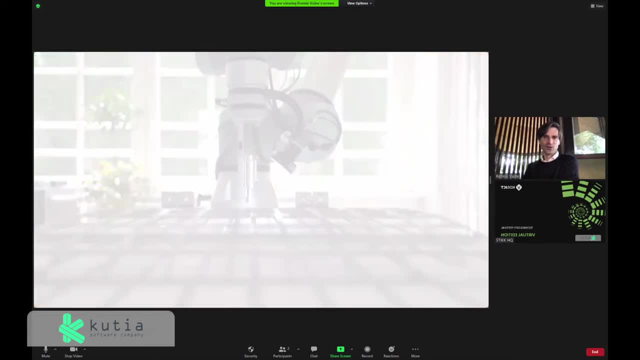 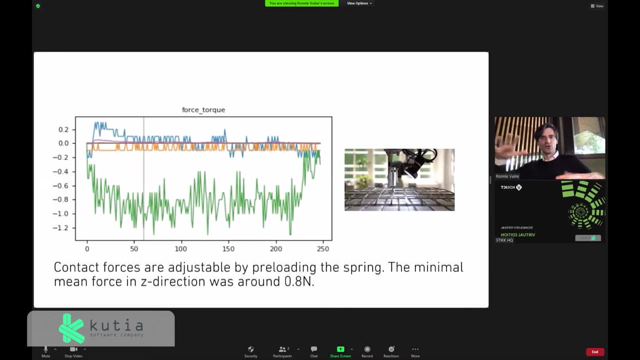 So this is how the application looks. It's very important that we do not touch this very fragile structure with more than a mutant of force, And the whole thing in reality is like seven meters long, So if you touch it only slightly, it will deform and wobble. So attempts to just make it look like it's not moving. So if you touch it only slightly it will deform and wobble. So attempts to just make it look like it's not moving, And then we can measure where everything is doomed. 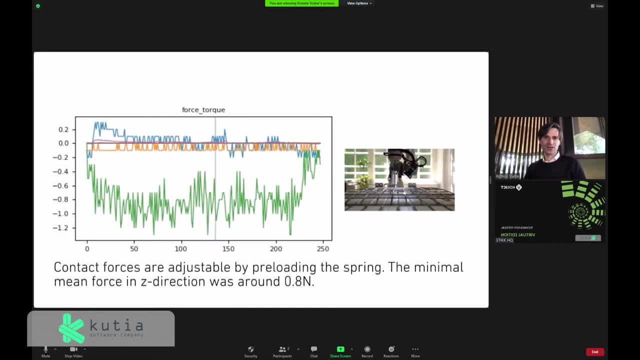 You sort of need to do this dynamically, And that is what we trained the robot to do in this case. Right now you're just looking at a diagram that shows we really We stay beyond one Newton of force that we may apply to that thing without breaking it. 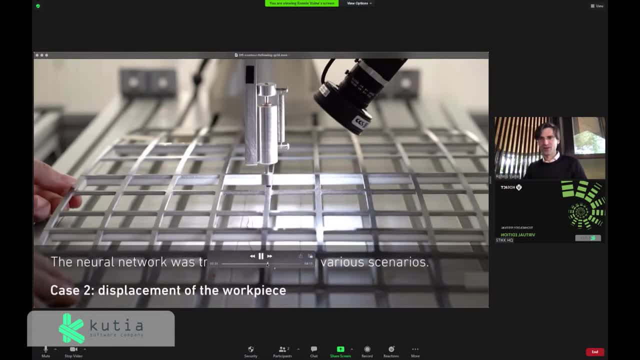 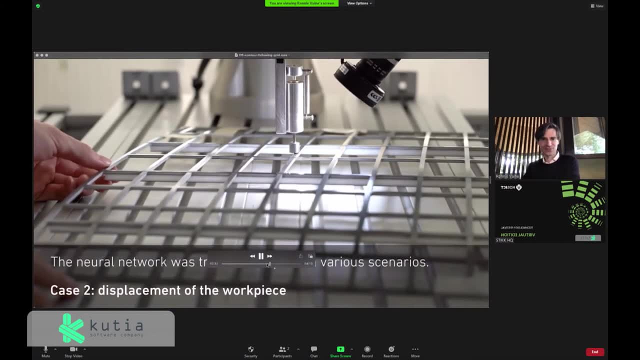 And I'll just let that. I think there was some noise that may indicate that we have questions, and I'll just leave that running in the background while we're answering the questions. Okay, so I think I'm ready. Okay, thank you. 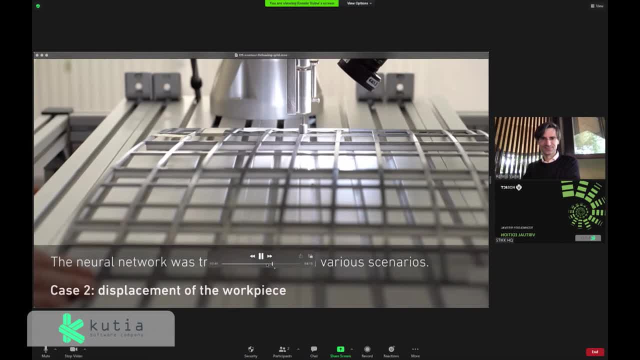 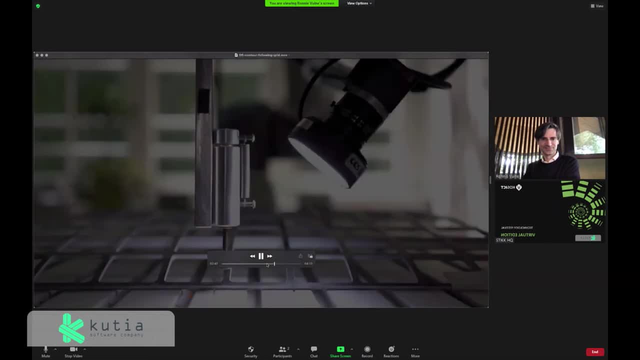 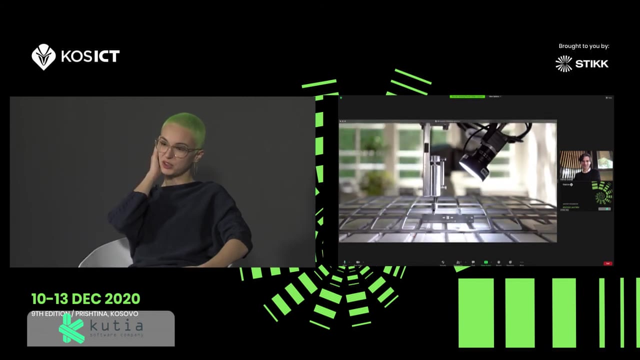 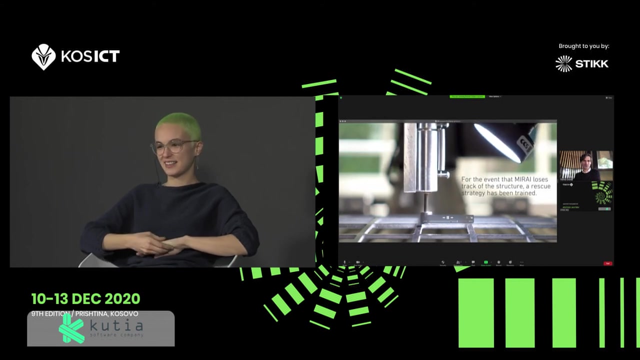 Yeah, Yes, Mr Vuyn, For the moment we don't have any questions, So if you can continue with your presentation, I will make sure that we'll get back to you. Okay, yeah, I'll just continue showing some of the material that we've done and explain. 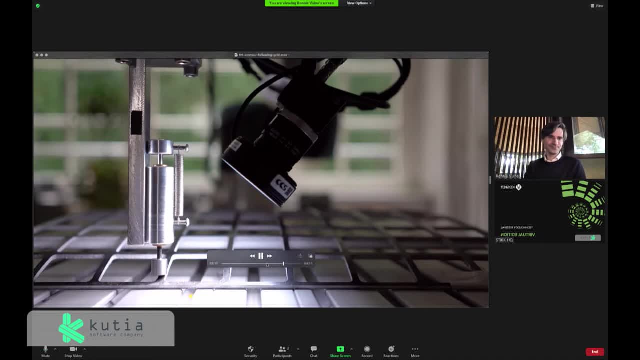 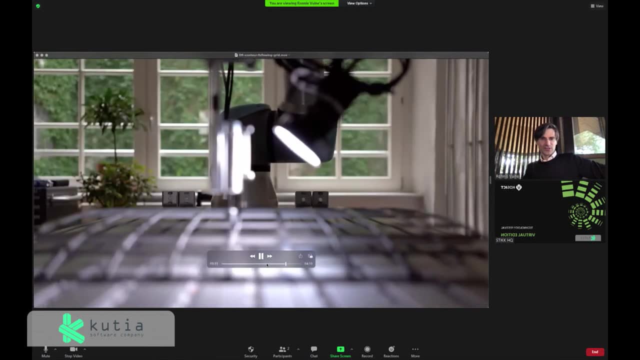 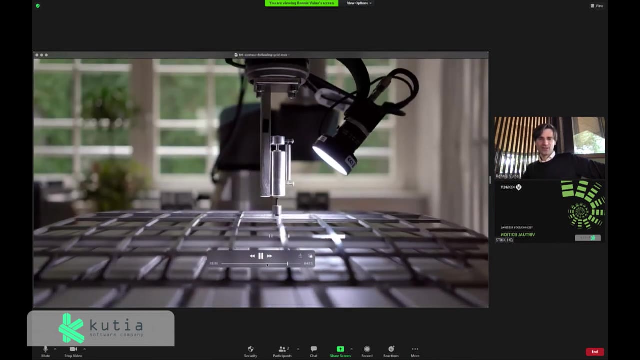 what you're looking at. So, yeah, what we're doing here is we're essentially showing that this trained robot pretty much works, even if you disturb it massively. And it also would work, if you know, if you imagine the whole workpiece. 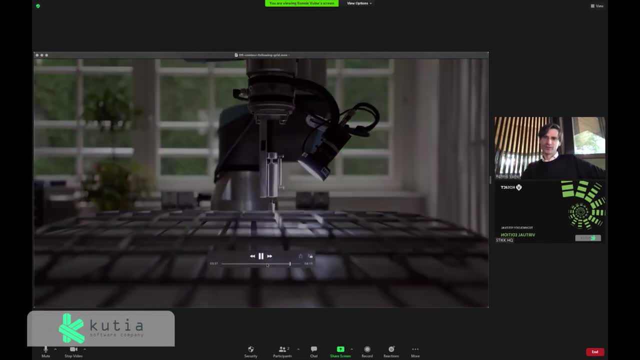 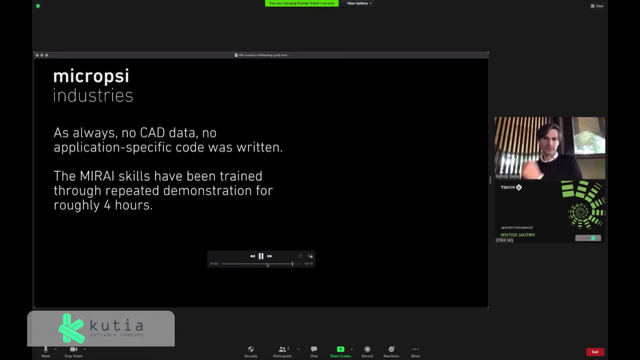 to be seven meters long. You could imagine putting the robot on wheels and just rolling it up to the workpiece, putting it anywhere, and then you could just start and do the work on that grid structure. So again, measuring is completely you know, wouldn't work in a case like that. 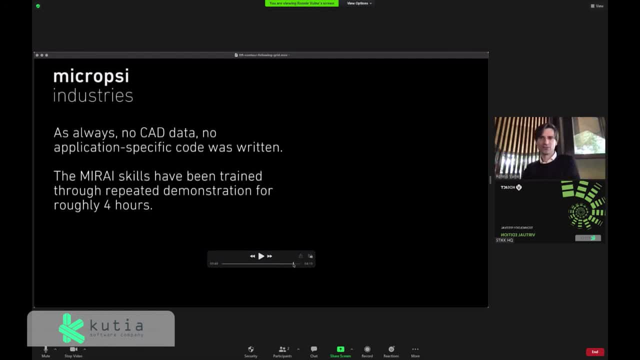 So we have- no, we don't even have- a 3D model of that, of that workpiece. Also, there was not a single line of code written. it's really purely a neural network that has been trained, that sits inside our product, Mirai, that creates those dynamic movements. 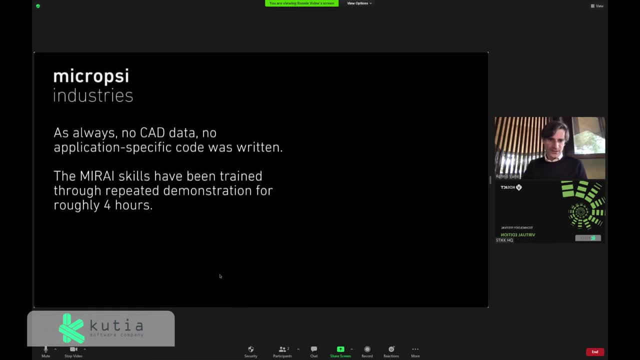 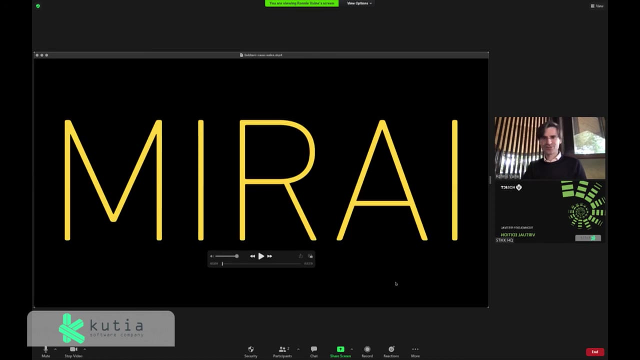 to handle that, to handle that part. And then let me show you something that we did for- I think I mentioned this earlier- that we did for a factory making refrigerators in the south. Okay So, Okay, So, let me jump ahead. 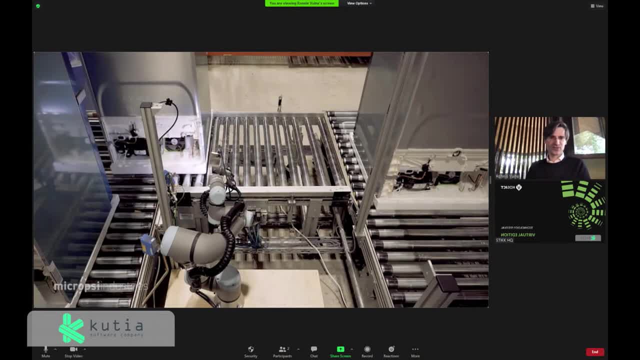 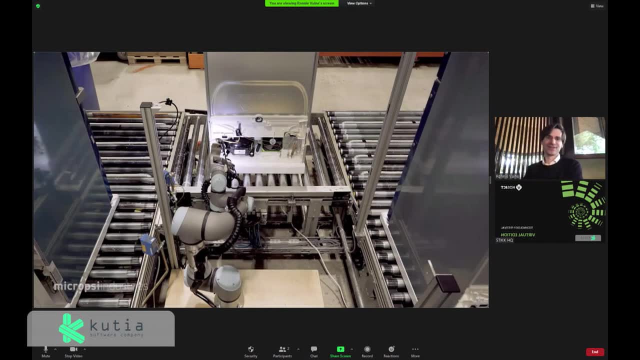 So I'll explain the problem. I'll stop the video and explain the problem when the fridge is delivered. So you're looking at the backend of a refrigerator here and you can see. I hope your resolution is good enough. You can see these copper tubes where coolant circulates. 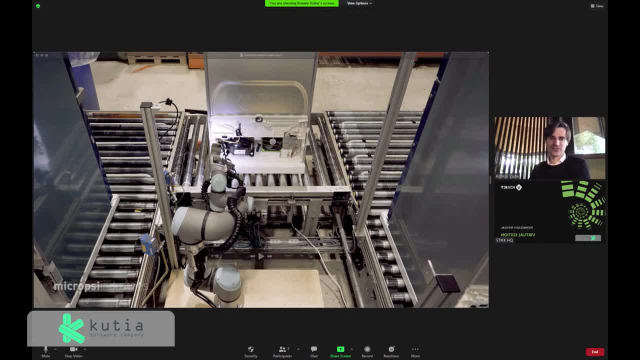 In the, in the, In the refrigerator and it's, you know, sort of compressed by this compressor here And all these copper tubes have been put in by humans. just a guy sitting 20 meters to the left of where we're looking at right now. 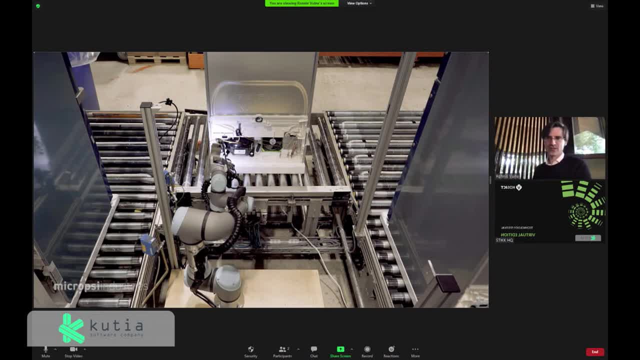 And they have put in those copper tubes and soldered them shut and then put coolant in. And the problem is, if one of those solder joints is leaking, then two things happen. First, your fridge stops working, And this is a high quality fridge, so it's you know. that shouldn't happen. 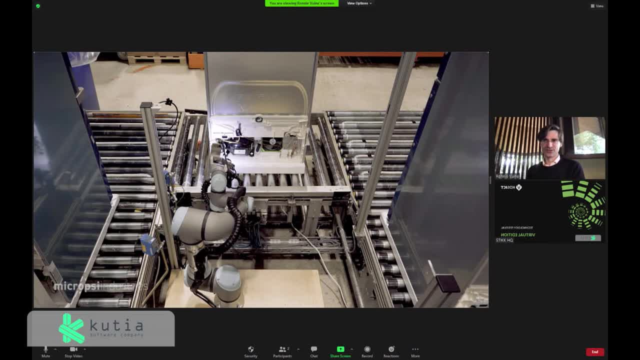 And also your kitchen explodes because the coolant is a lighter fluid. So you really want to make sure that those solder joints are in proper order. So what today happens is somebody uses a manually led probe. it's like a little artificial nose that you need to bring up to within one millimeter of the solder joints to see if it can sniff. 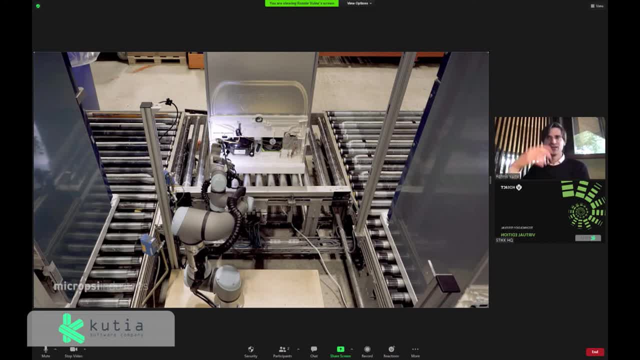 out any coolant molecules In the air around the solder joint, and that's, of course, extremely boring work that nobody wants to do And people get sloppy after a while. So the factory has tried to robotize this for quite a while. 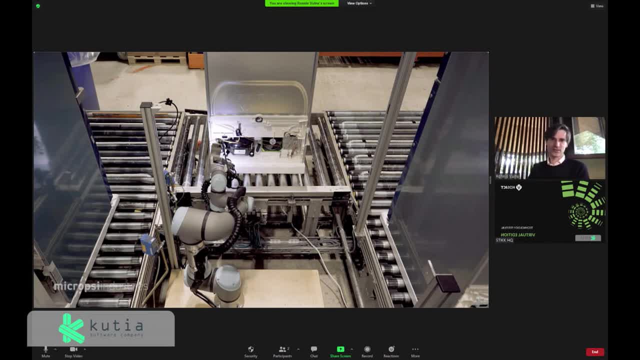 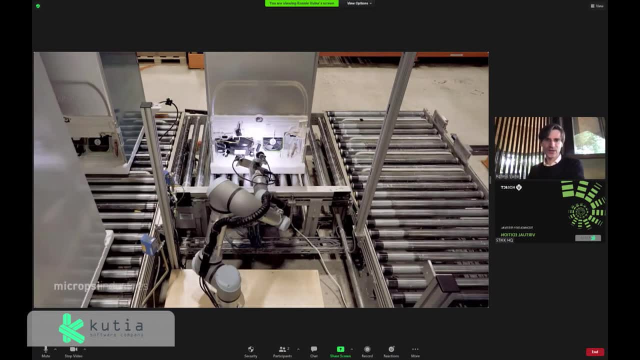 And this is essentially the first working solution that has been created through the introduction of trainable AI. So what you see happening here is: the factory delivers a fridge, It gets stopped in front of the robot, And then these forward movements as we move those. 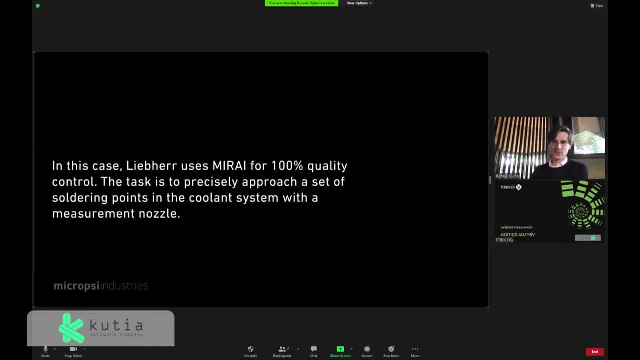 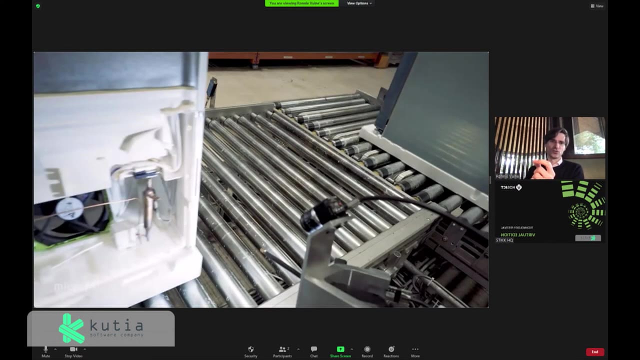 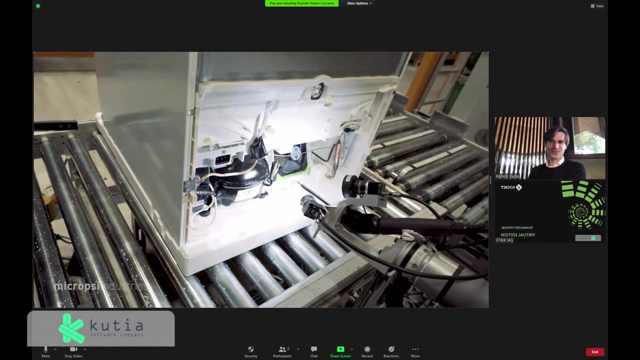 These Fridging this sniffing probes towards the solder joints. This movement has been trained using AI, using our product to find the closest point that the sniffing nozzle can get to the solder joint. Sometimes it even touches it. The solder joints are always in slightly different places and they always look slightly differently. 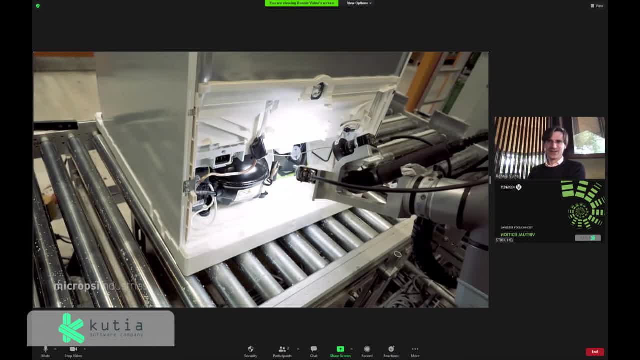 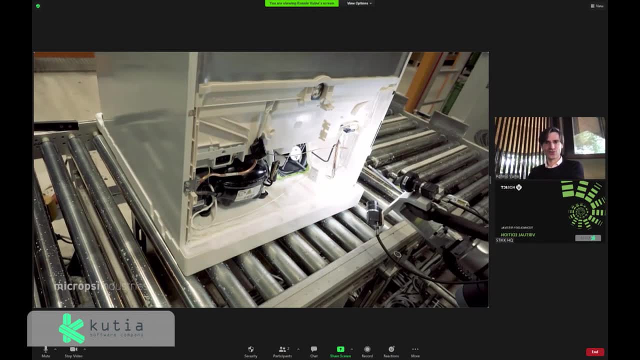 They have been built by hand. depending on who does the soldering, they look very corroded or they look super clean, or there's a drip, you know there's a drop of solder fluid on it. So both the position of the solder joints varies. with like five, you know, within a 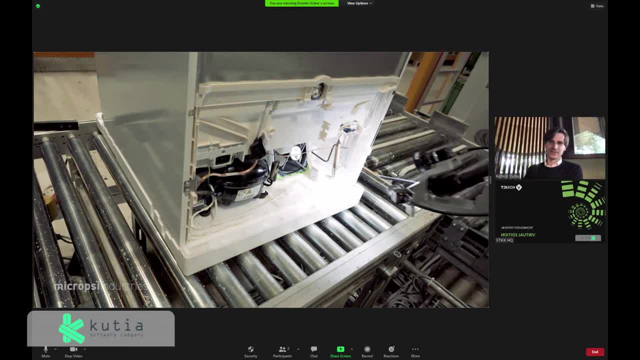 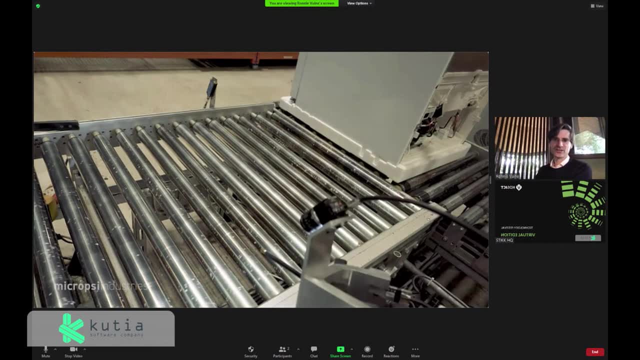 sphere of like five centimeters, And the look of the solder joint really varies and you need to use cameras and AI to pick up where they are and guide the robot there. And that's what we did here. Yeah, that's what the system sees. 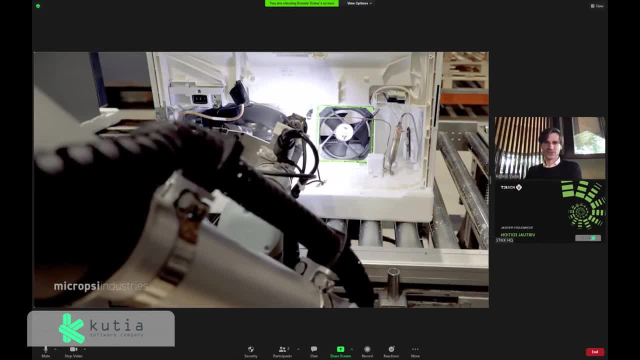 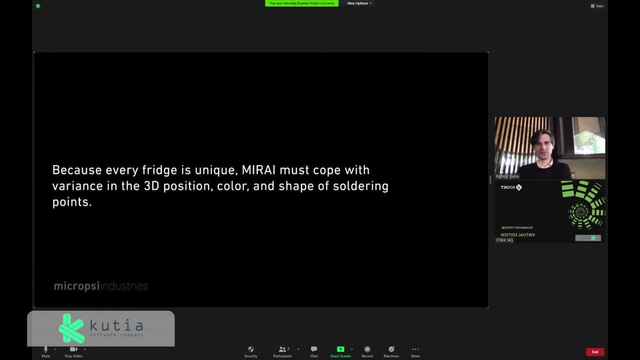 So we're even going, Okay, Going- around some of those copper tubes in some cases- And again, this has not been, you know, custom built for this customer. It has been trained on site in that factory. We weren't involved. 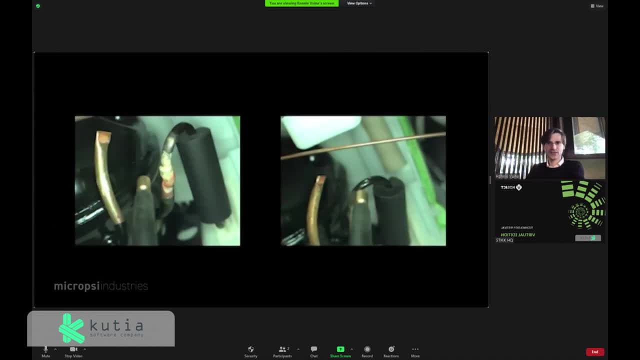 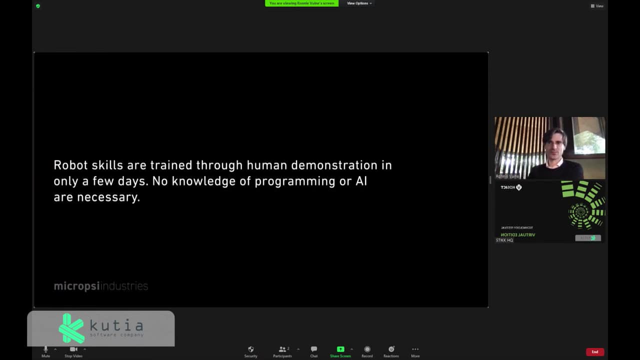 Okay, We were involved with helping build a system, but we didn't do the training. Training has mostly been done by local staff that worked in the factory and showed, by guiding the robot by the wrist, how a good movement looks like, And then it generally. this is the guy. his name is Siggy. 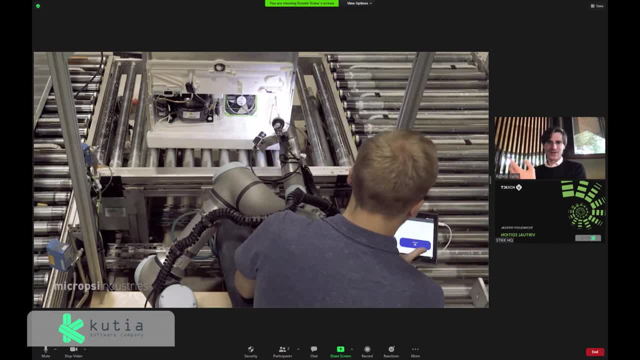 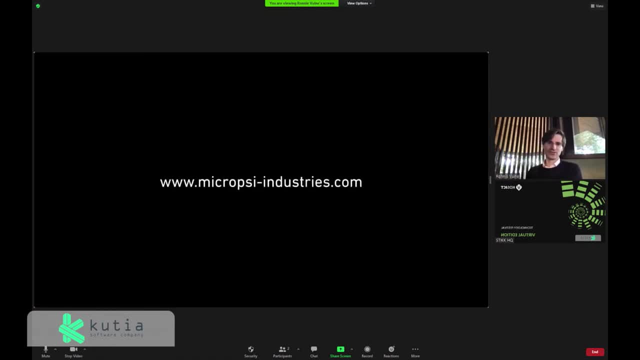 He does the training here And our system generalizes over the demonstrations he gave and then knows how to move relative to the fridges, depending on what it sees. Okay, let me see if I have one more. That's interesting enough. 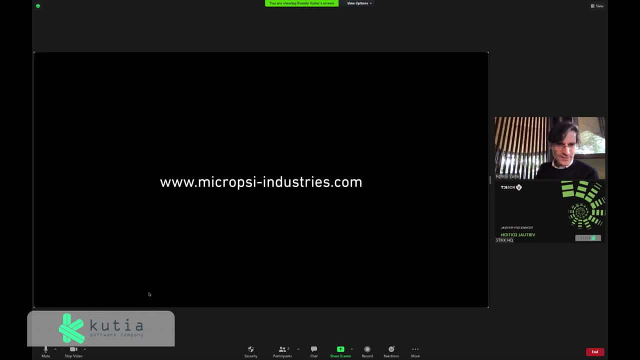 Yes, Do I have the? No, I don't have to car charging, So I'll just do cable plugging. Oh yeah, need to share the. This is one of the earliest things we did, where you can also quite neatly see the real. 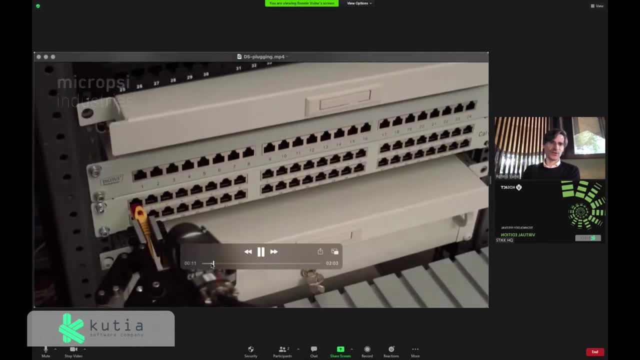 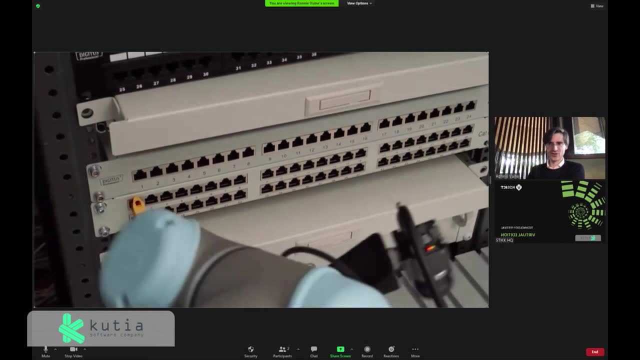 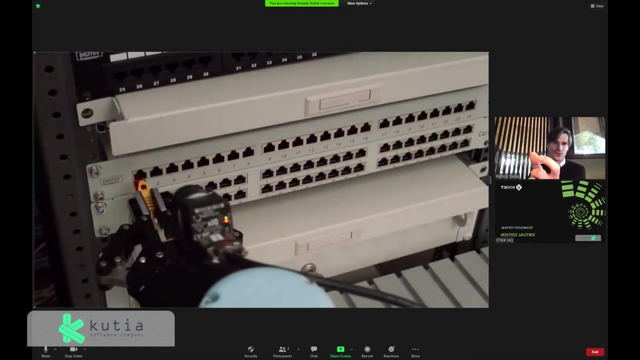 time properties of the system. So what we're doing here is we're plugging in ethernet cables into a patch panel. Of course the system knows where the cable needs to go, right. So the AI part is just finding the insertion point right. 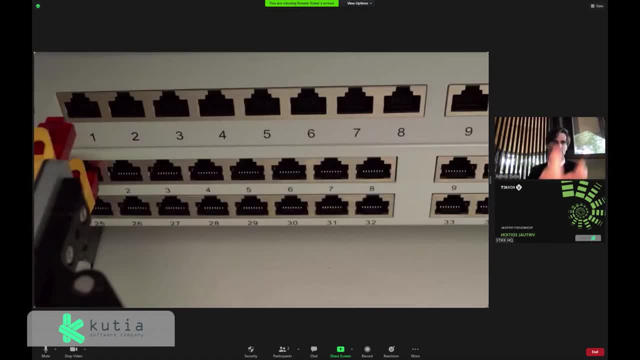 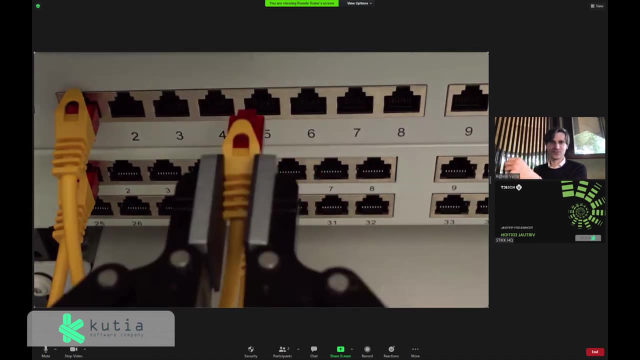 If you, there's a little slightly off when the algorithm drops the robot in front of the point of the slot that we want to plug in and then the AI takes over the real-time control for making this sort of tender force responsive. Okay, 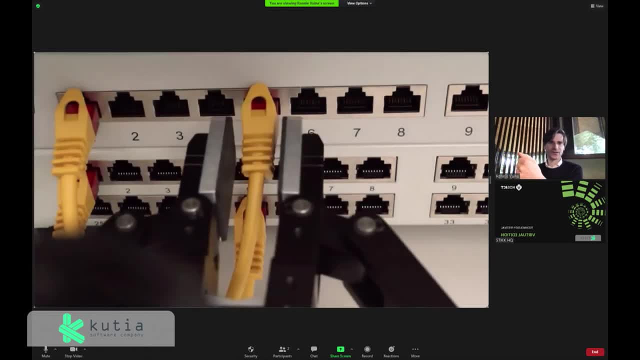 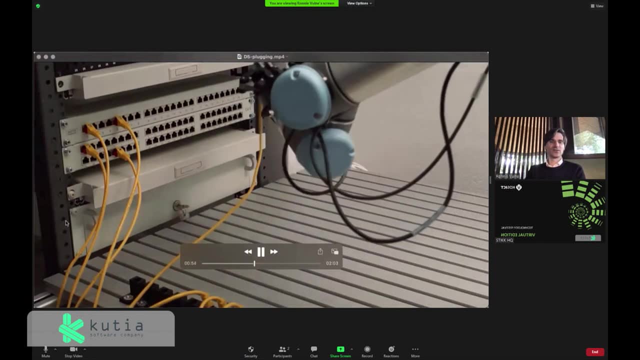 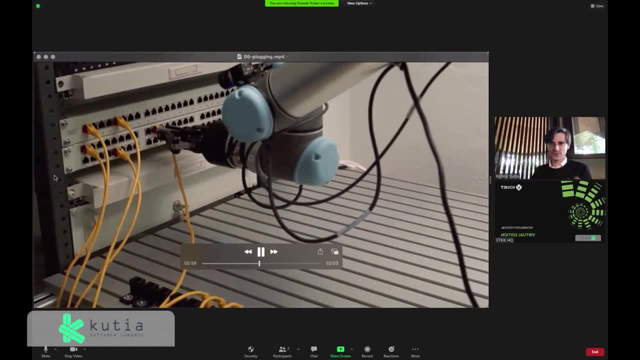 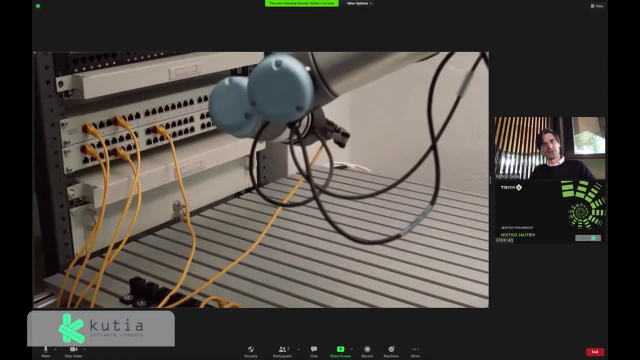 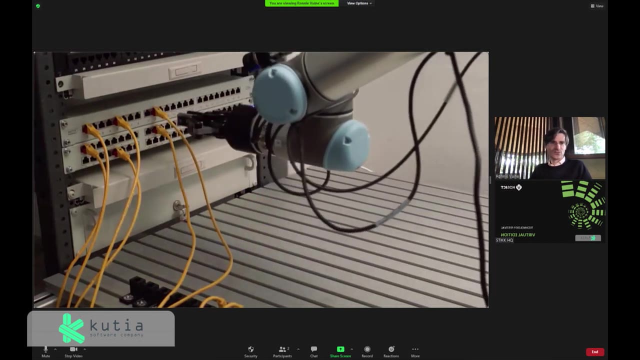 how the whole 19 inch rack is positioned in the actual factory. it came on a Euro palette So it was never precisely aligned. You can pick up these cables from from a desk where they have been provided And properly and safely insert them to wire a 19 inch rack. 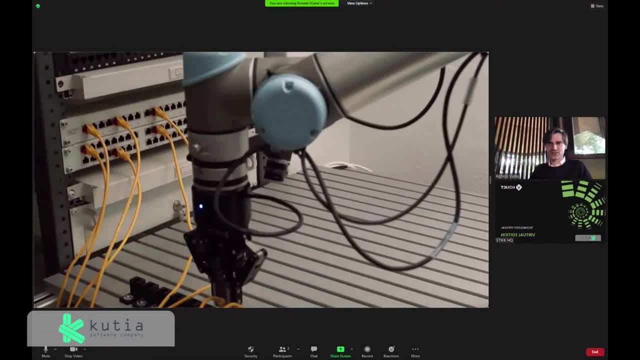 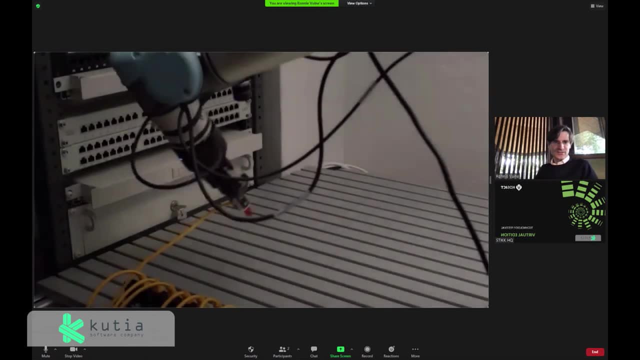 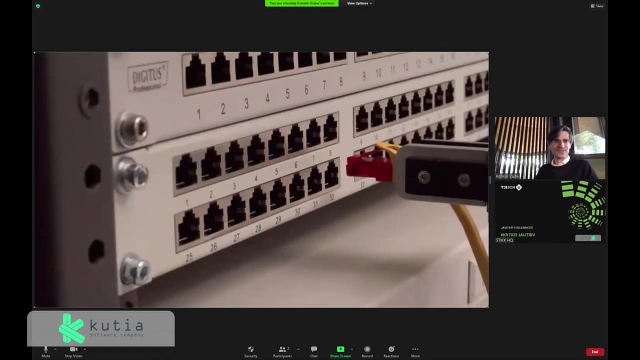 19-inch rack that goes into, I think, a data center- for I believe Microsoft was the customer in this case- And we use this application to demonstrate that it's actually real-time. You can mess with the robot quite badly as it moves right, So we just hit this and then it still. 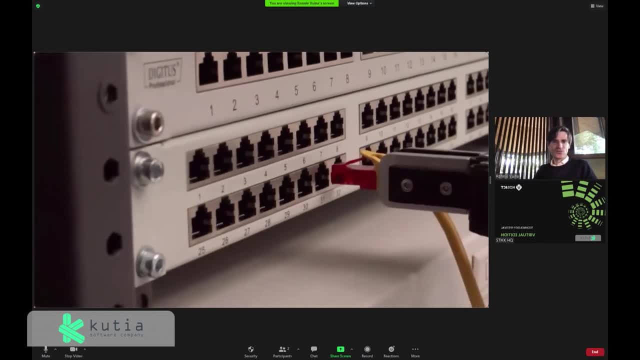 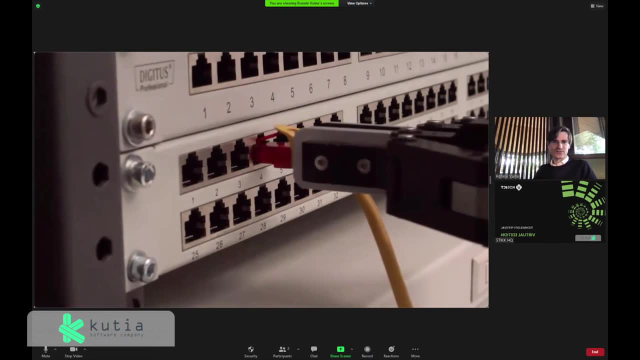 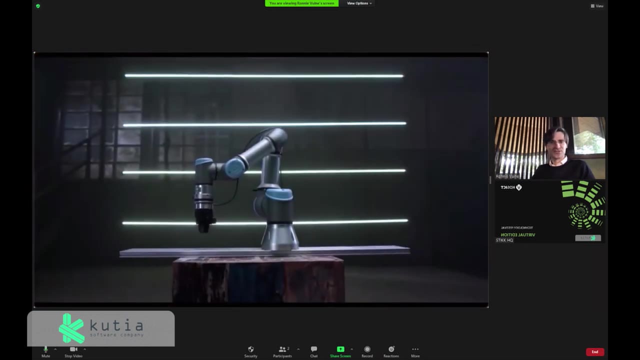 plugs in So you can even, as it moves, try to confuse it, and it just wants to get this plug into where it needs to be, And this is what we did mostly in the early days, which was confusing and annoying robots. We were always wondering whether they would fight back at some. 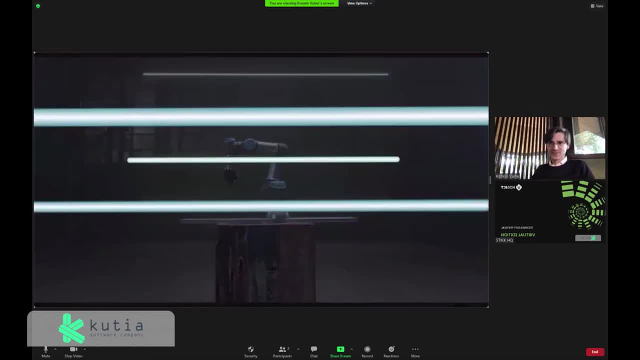 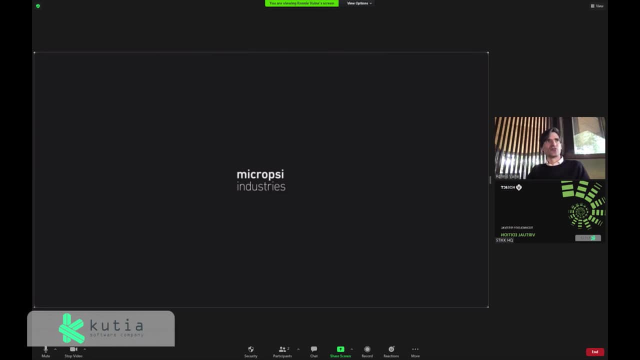 point. Okay, so I think that gives you what I know about the industry, where it is and what the interesting fields are at this point, And it shows you some of the things that are possible today in the fields, Well, in the field of robotic arms, Okay, so that really concludes my part. I believe, if there